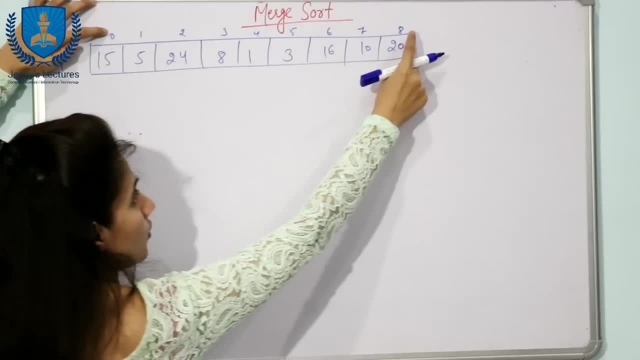 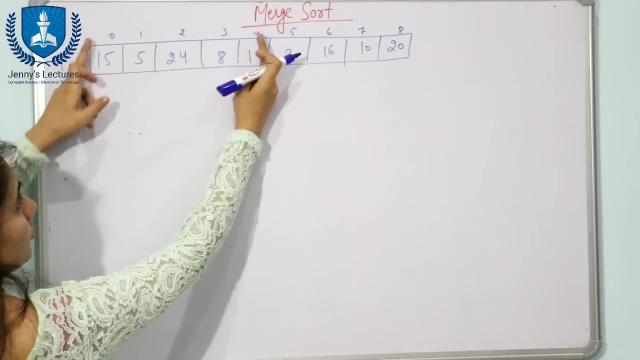 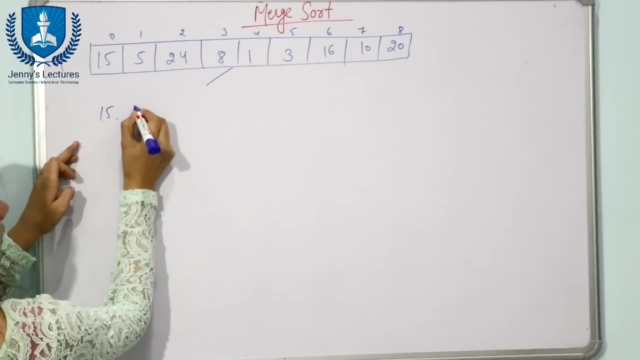 So we are going to take some sub inventory as defaultInterpreted low position. So what that means is we are gonna get a four by four sub array of three. So we are going to divide this sub array into two equal sub arrays. We're going to Alors one over. 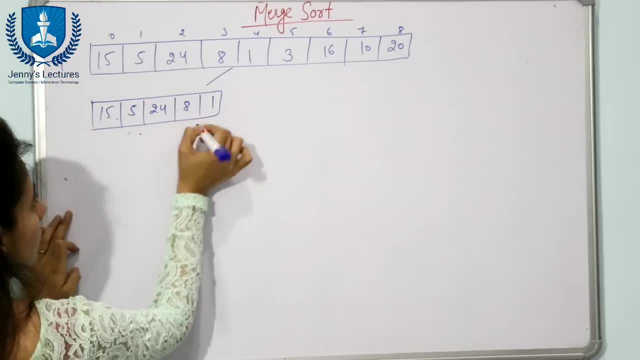 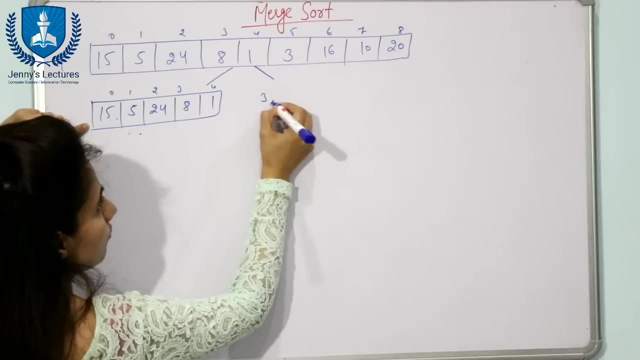 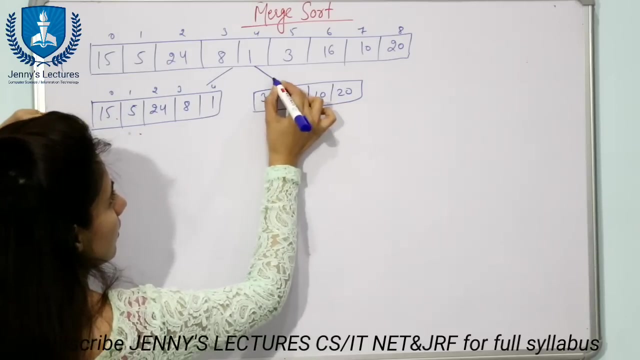 So what if that Due zero plus eight C is zero? slower bound: This one is your upper bound- is zero plus Eight is 88 divided by two. that is for. So in four, six, zero to 4.. And from 5 to 8, we are having another sublist. 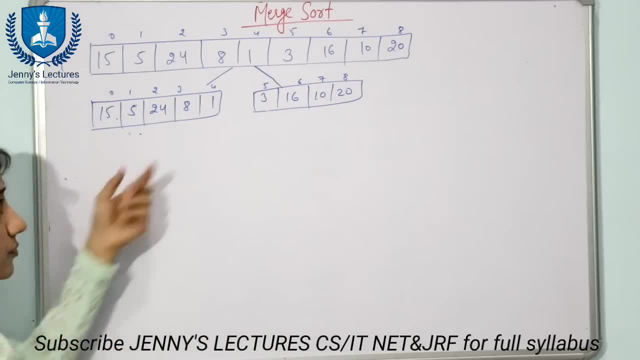 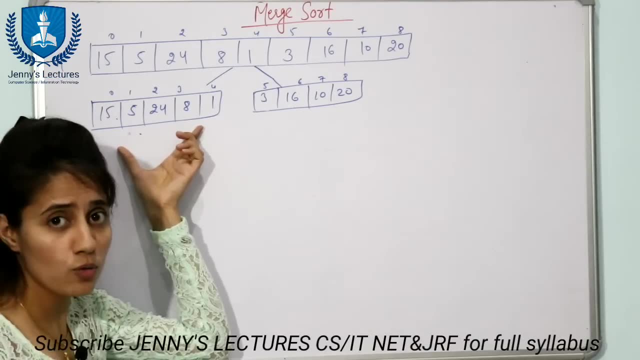 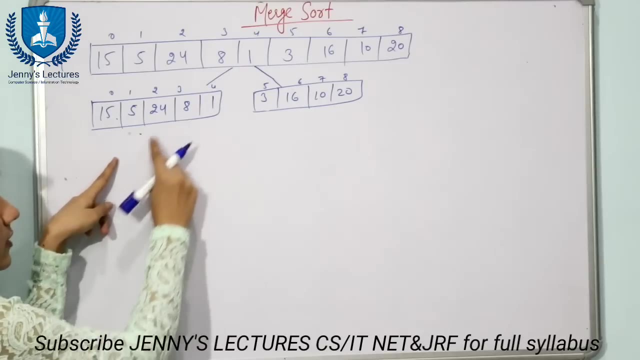 5,, 6,, 7,, 8, like this. Okay, Still, this sublist is having how many elements? 5 elements, But we are going to divide the sublist till we get a sublist having 1 element. So we are further going to divide the sublist. 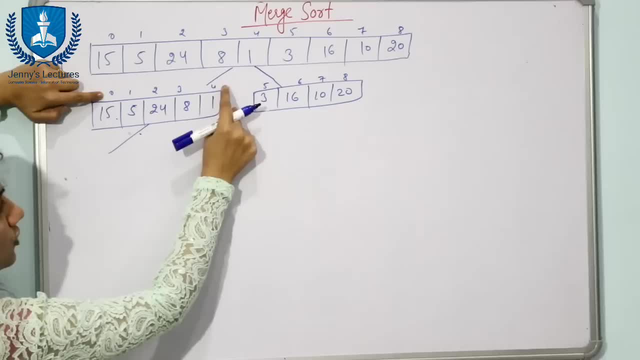 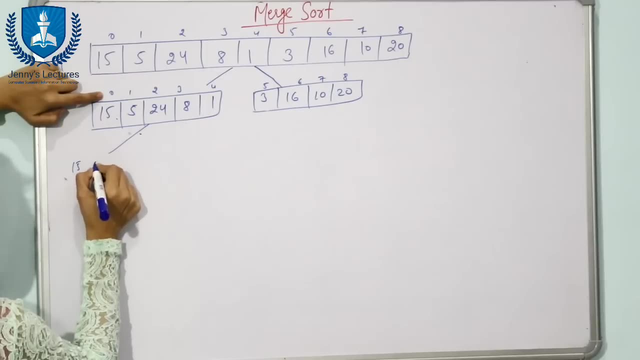 Okay, Into 2 halves: 0 plus 4,, that is 4,, 4 divided by 2,, that is 2.. So middle position is 2.. From 0 to 2,, 15,, 5 and 24.. 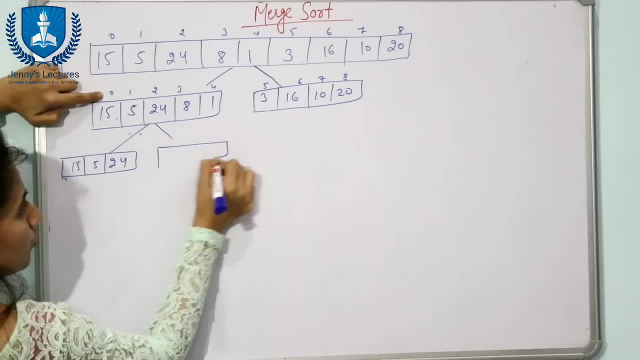 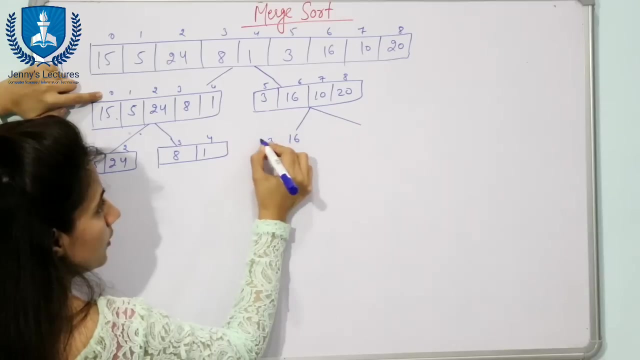 This is one sublist, and another sublist would be 8 and 1.. From 0, 1, 2, here we have 3 to 4.. Right, This will be again divided into 2 parts, And 3, 16 would be 9.. 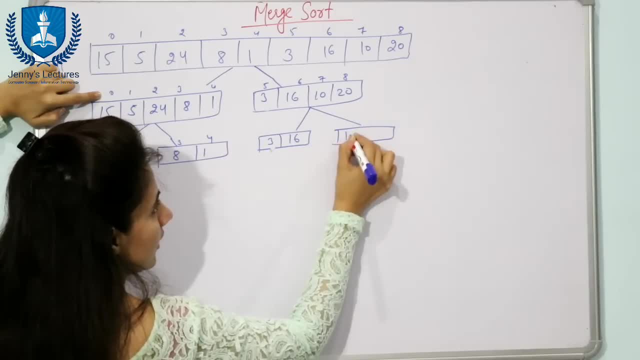 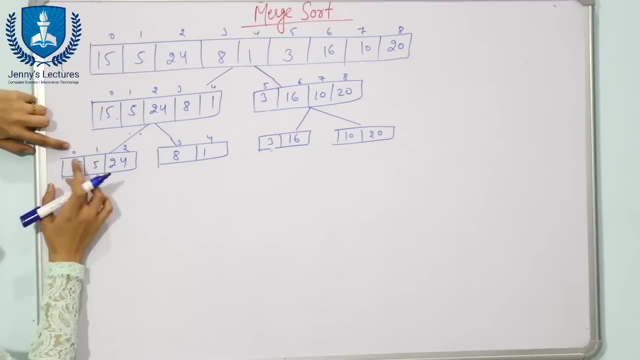 So this would be in one subarray And this 10 and 20 would be in another subarray. Fine Again. this list would be divided into 2 parts. Middle is 1.. 0 plus 2 is 2.. 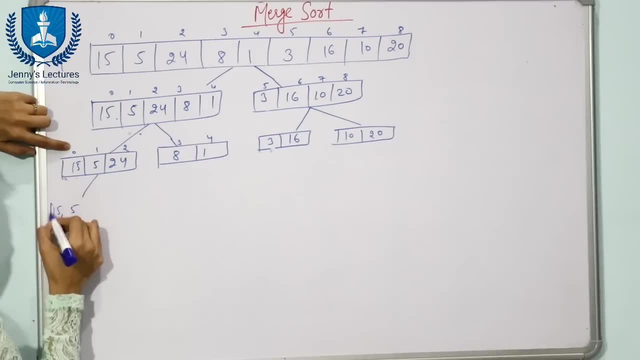 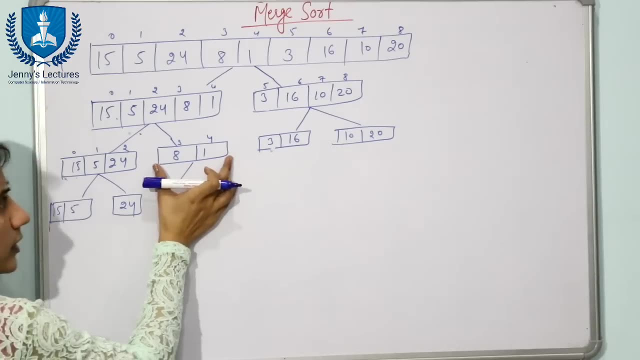 2 divided by 2, that is 1.. So 15 and 5, this would be in one list And this 24 would be in another list. Same: this would be divided into 2, halves, Fine, And this would be 8 and this would be 1.. 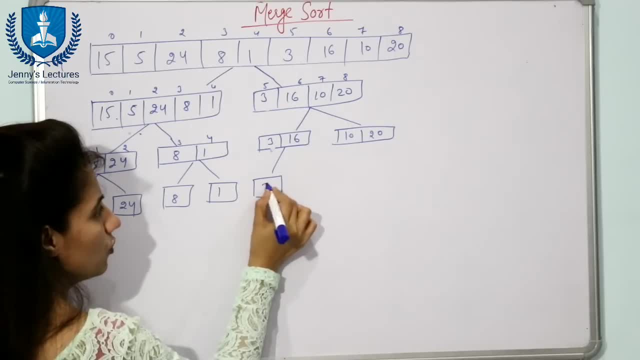 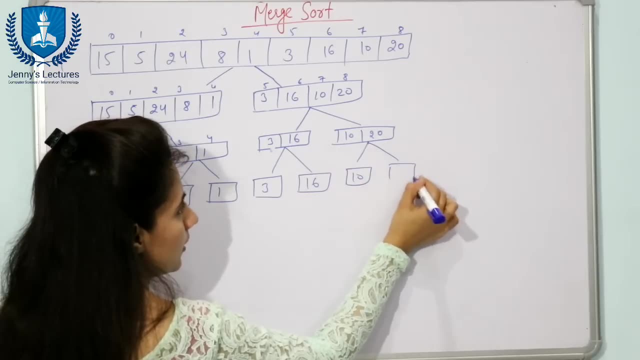 So this one sublist would be having 1 element. This would also be divided into 2 halves. 1 is having 1 element 3.. 1 is having 1 element 16.. Here, 1 is having element 10 and 1 is having element 20.. 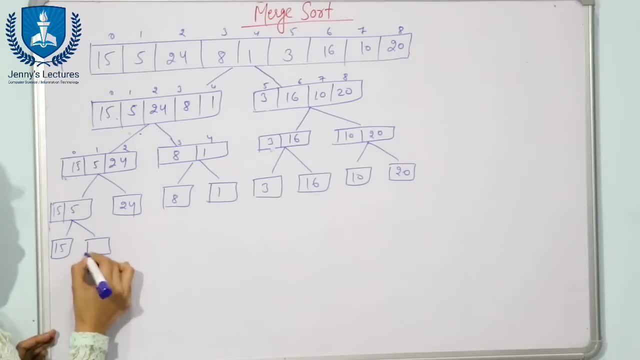 Now this 1 is having element 15.. Another is having element 5.. Fine, Now we cannot further divide these sublists. Why So? because each sublist is having only 1 element, And that is the condition. you have to stop dividing. 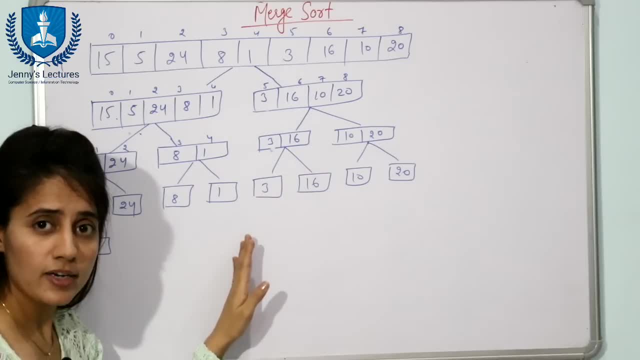 You will keep on dividing the sublist. You will keep on dividing the sublist until each sublist is having only 1 element. Now, each sublist is having only 1 element Now. next second step was: you have to merge these sublists. 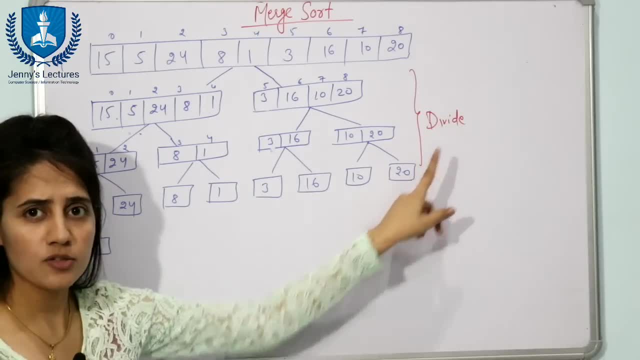 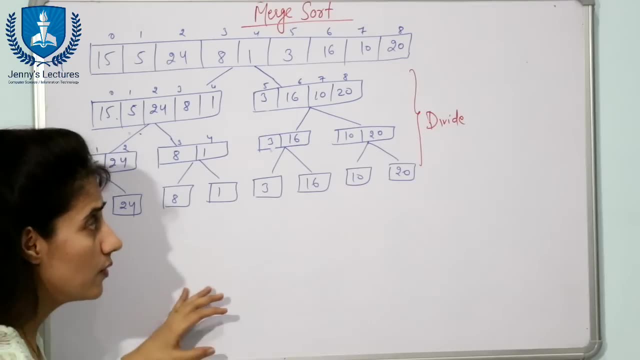 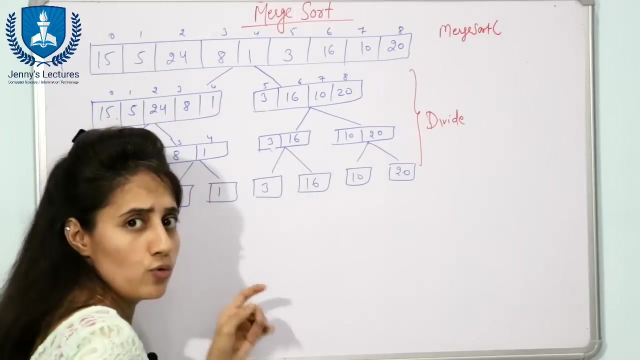 So now till now, this divide. the first step is over. Now second step is: what for Merging? Okay, Now, if I write down the algorithm, then how you will write, See Merge sort. we are going to take a function: merge sort. 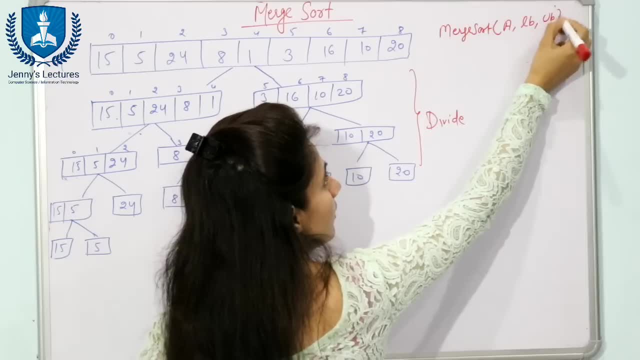 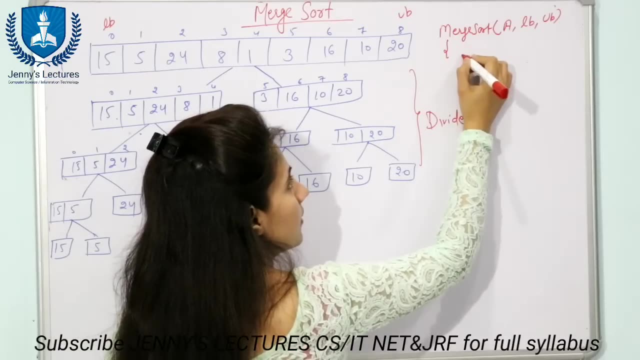 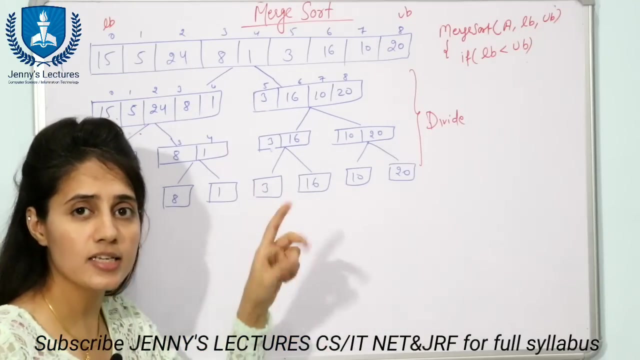 A is array. We are going to pass lower bound and upper bound. This is lower bound and this one is upper bound. Right, And if lower bound is less than upper bound, it means at least that array is having 2 element. Lower bound is less than upper bound. 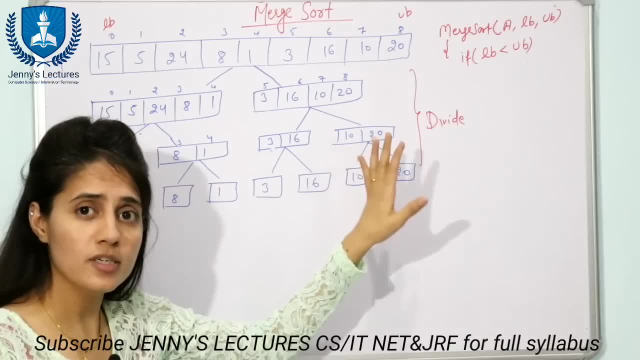 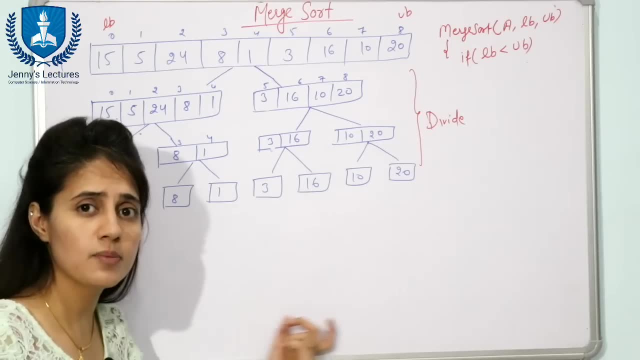 If 2 elements are there, If 2 elements are there, then you are going to divide these sublists, Right. And then you are going to divide that particular list into sublist, Okay, And then each sublist is having only 1 element. 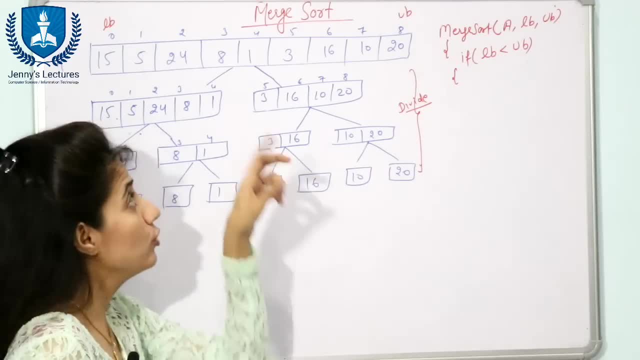 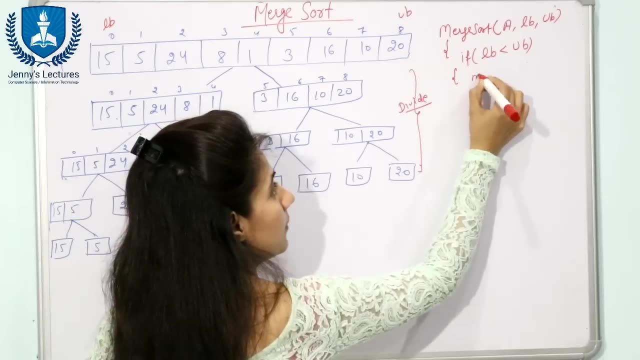 So now, if this condition is true, Now next is we are going to divide the array into 2 halves, equal halves. So for that thing you have to calculate mid element. How to calculate mid element? Mid is equal to lower bound plus upper bound divided by 2.. 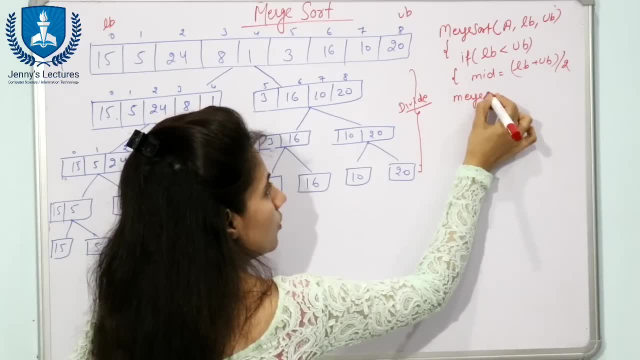 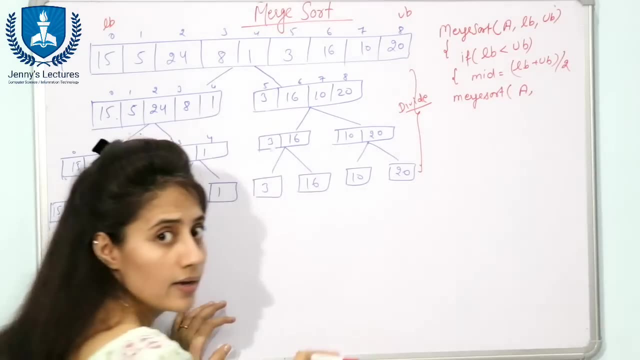 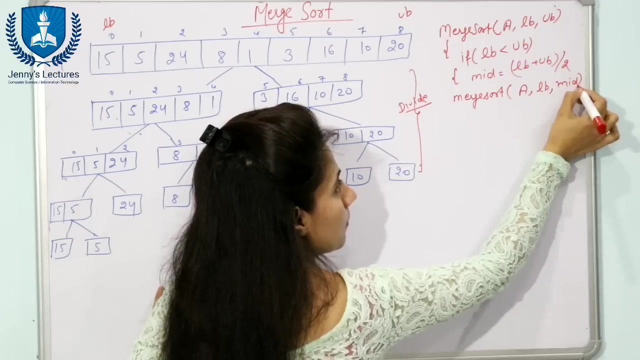 Fine, Now we are again going to recursively call, Recursively call, merge, sort on array A and from lower bound to mid, See from lower bound 0 to mid. Here, mid is what 4. Because 0 plus 8.. 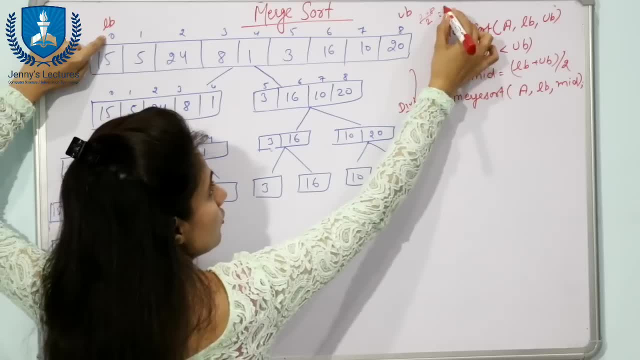 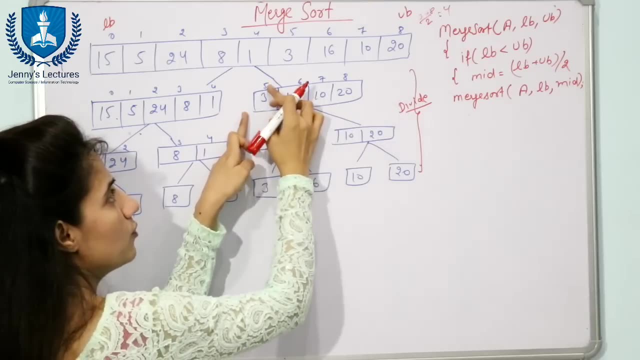 0 plus 8 divided by 2, that is 4.. So mid is equal to 4.. So one half is from 0 to mid, And next half is from 0 to mid And next half is from 5 to 8.. 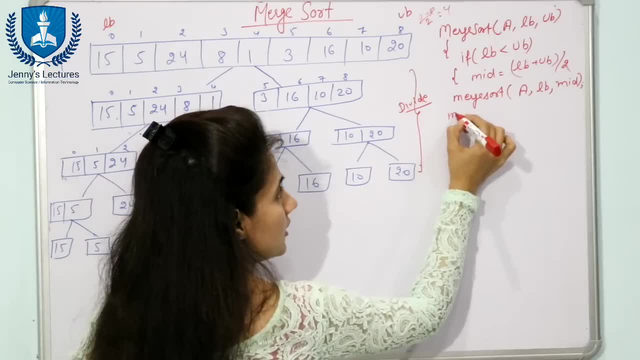 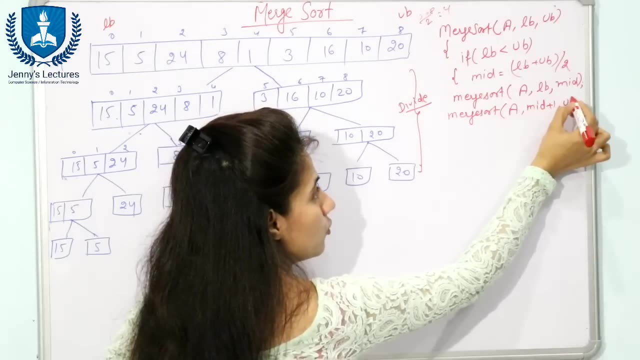 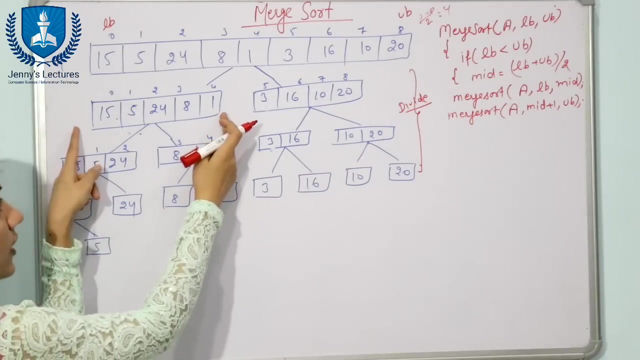 That is mid plus 1 to upper bound. So next is merge sort on array A from mid plus 1 to upper bound Right, And this is what Recursive call. We are going to recursively Now again, we are going to divide this into 2 halves, from 0 to mid, mid plus 1 to this. 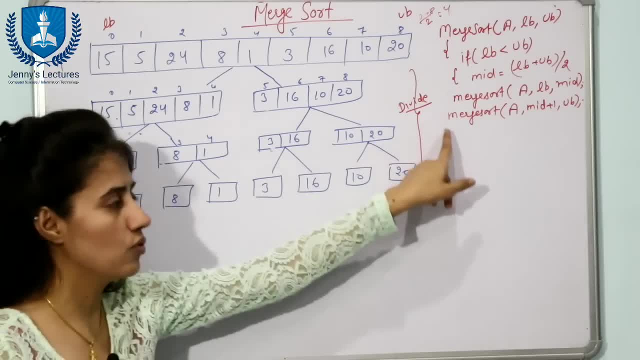 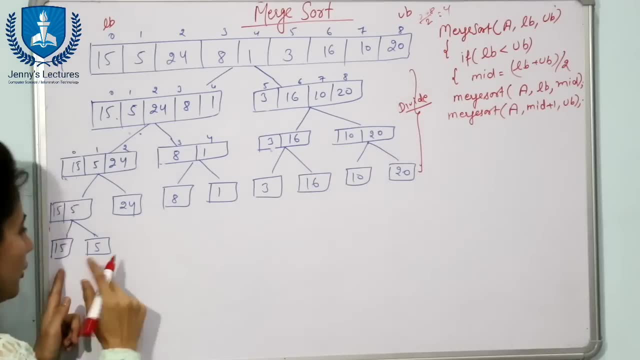 one Again, we are going to divide into 2 halves, So this is a recursive call To let us see To left part and to right part. Fine, Finally, after that, we are going to merge these arrays. 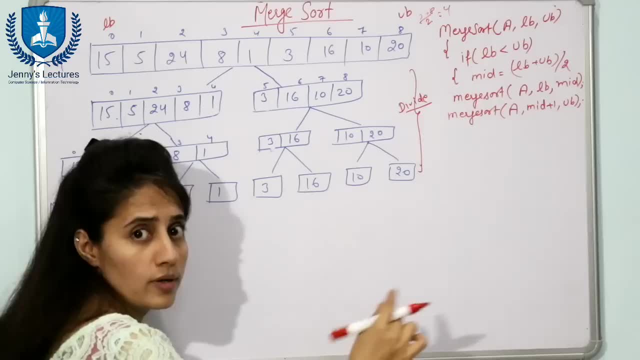 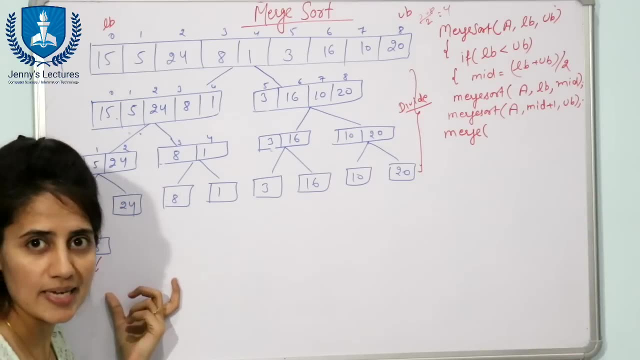 Fine, So after this merge sort, next next is what A method that is merge. We are going to merge these arrays. Now in merge, we are going to pass in array A. we are going to, we are going to merge. 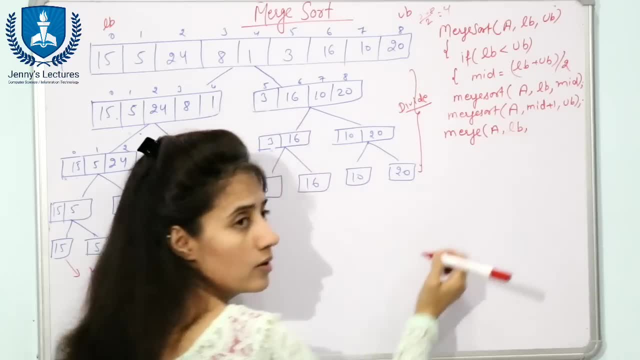 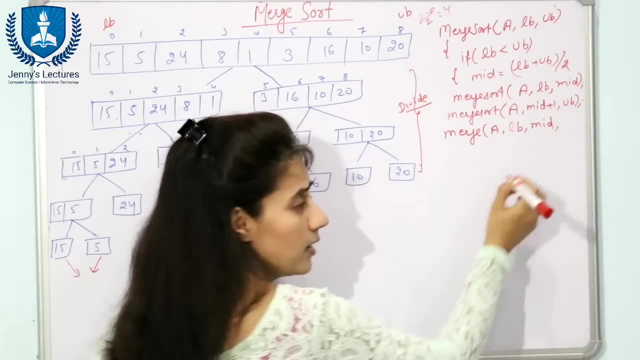 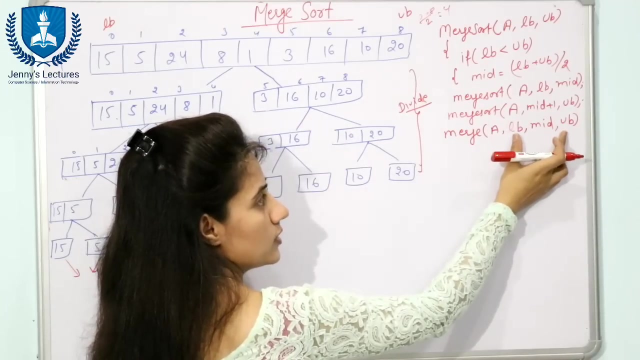 these 2 halves. So from Lower bound to mid. one half is from lower bound, lower bound to mid, and another is from mid plus 1 to upper bound, So from mid plus 1 to upper bound. So you are just going to pass these parameters: lower bound, mid and upper bound. 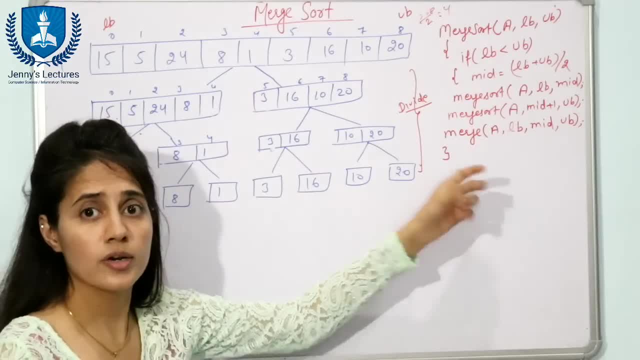 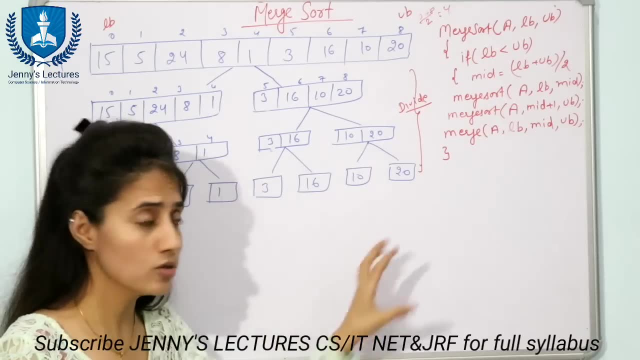 Fine, So this is the merge sort. Now, here, the main thing is: you have to write down the code for this merge function, That this backbone of this merge sort is this merge function, how we are going to merge these arrays. Okay, 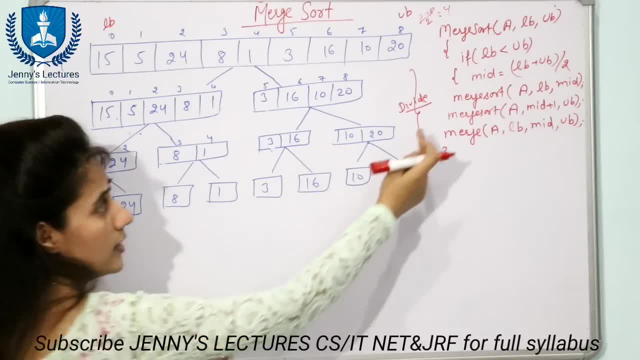 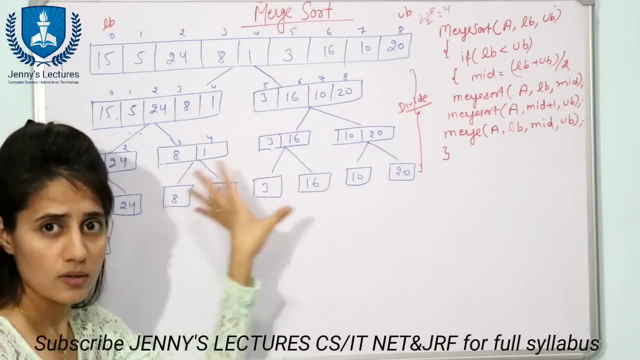 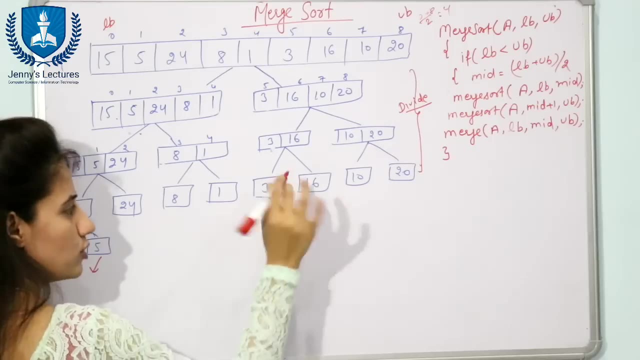 Now, if, if you are, this is the recursive call, Fine, This is recursive call. If you, if you draw a recursion tree for this, this numerical, then how you will draw: See. first of all, we are going to call merge sort. 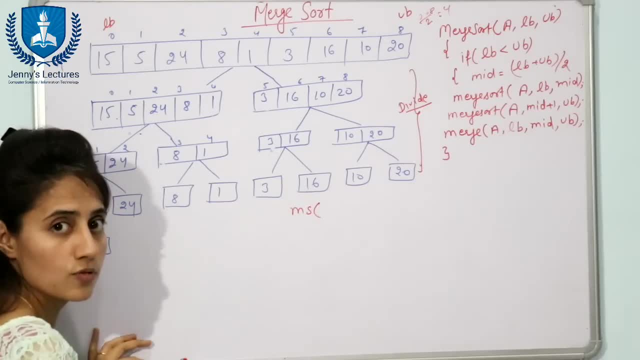 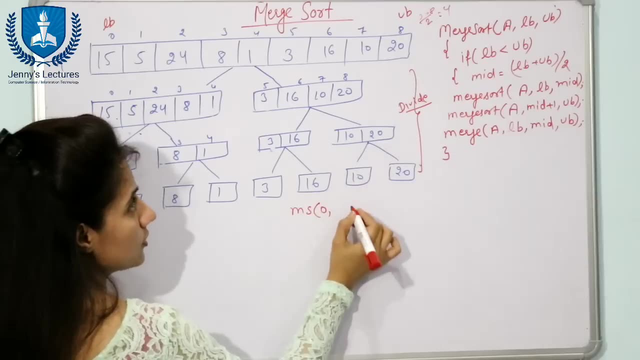 Suppose I am going to write ms only. Fine, Array a. I am not going to pass array. I am going to pass this lower bound and upper bound. Lower bound is 0,, upper bound is 8.. Fine, Lower bound is less than upper bound. 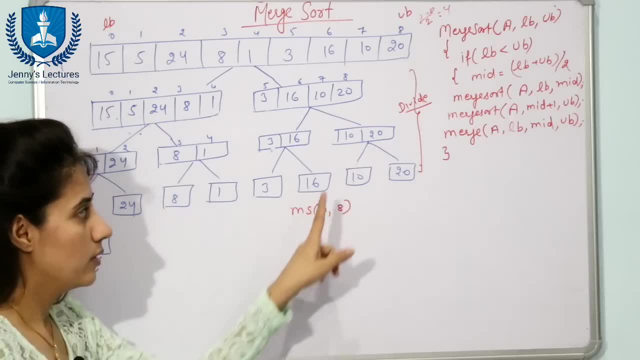 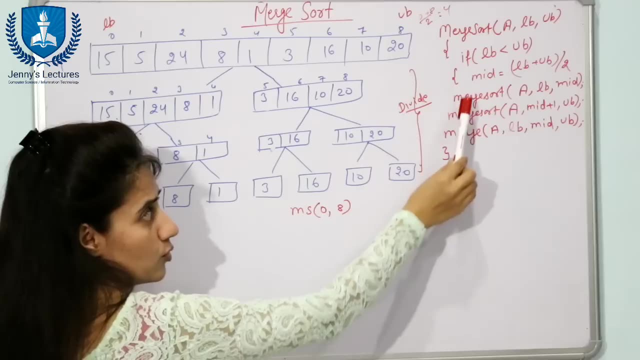 Yes, that is true. Then we calculate mid: mid is equal to 0 plus a divided by 2, that is 4.. Fine, Again, merge. three statements are there: This, this and this. So I am going to divide into this into three parts. 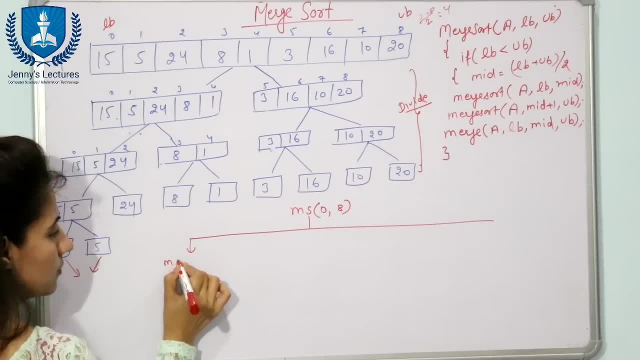 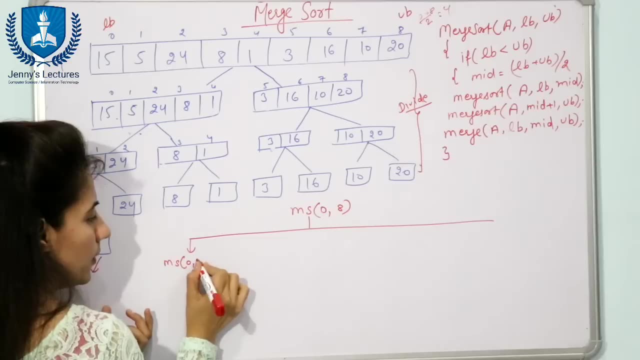 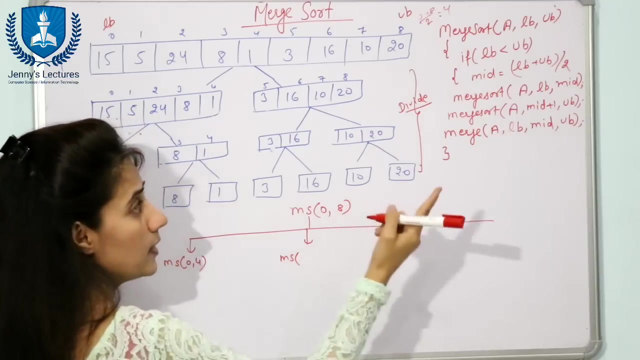 So here we have Again merge sort. Merge sort I am. I am going to write ms for merge sort: Lower bound to mid. Lower bound is 0,. mid is 4.. Fine Again. second is merge sort: mid plus 1.. 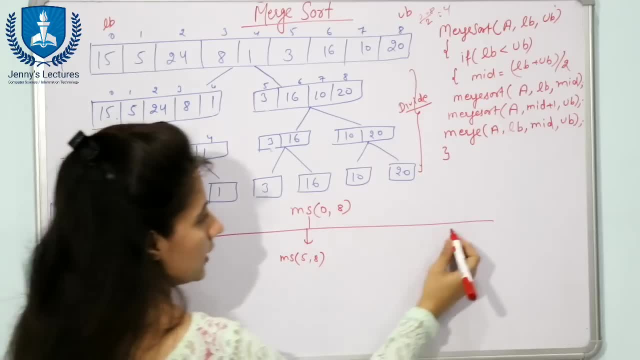 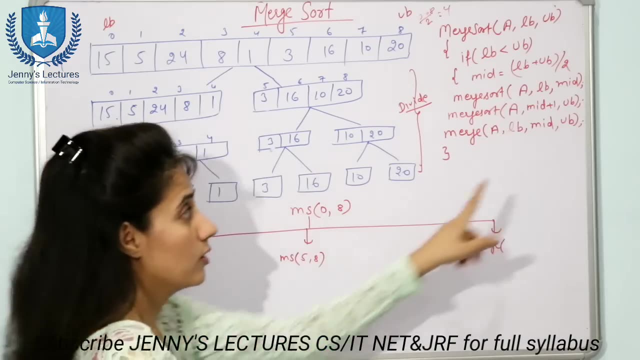 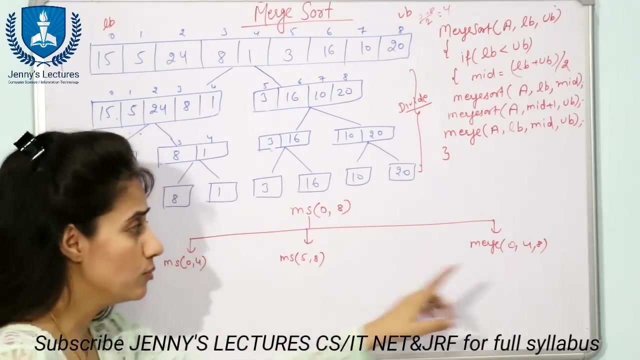 That is, 5 to upper bound is 8.. And next is this: merge would be. merge would be: lower bound is 0,, mid is 4.. bound is 0,, mid is 4 and upper bound is 8.. From 0 to 4 and 5 to 8, we are going to merge. 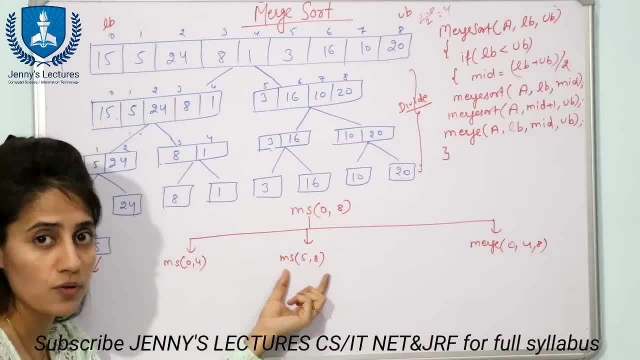 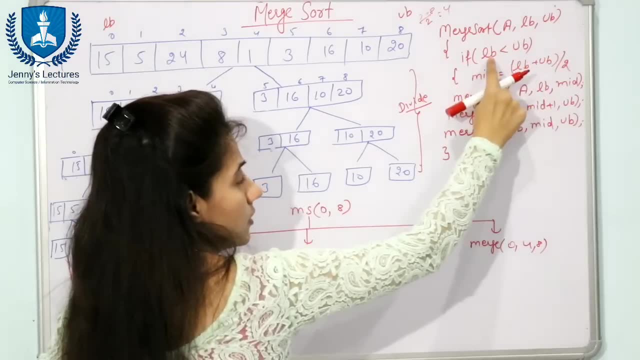 these arrays. But after sorting of these subarrays, fine Now from 0 to 4, again recursively merge. sort would be called from 0 to 4.. 0 is less than 4,. yes, Calculate mid. Mid is. 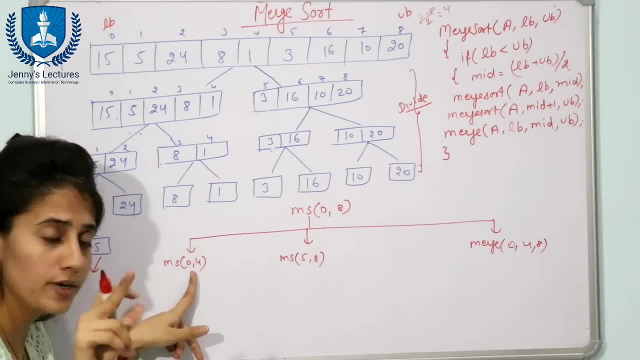 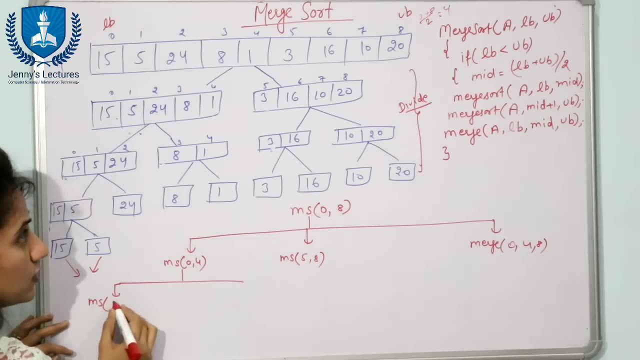 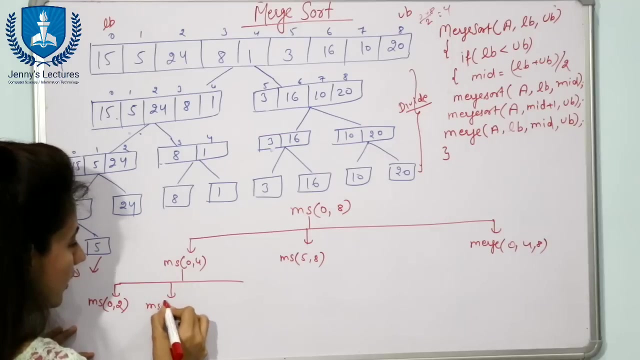 equal to 0 plus 4 divided by 2, that is 2.. Midpoint is 2.. Now again, call this: merge sort. Now see: M is 0 to 2.. Mid is 2.. Now, here again: M is 3 to 4.. Now, here we have. 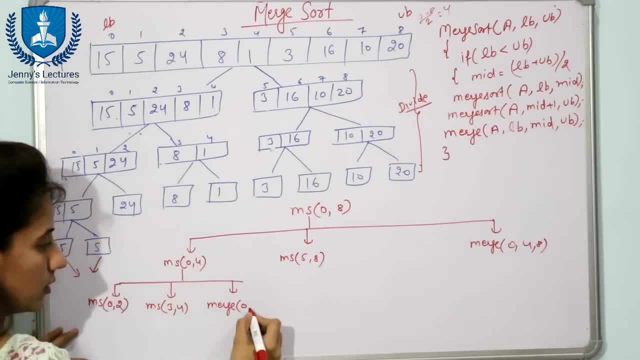 merge 0, then mid is 2, then mid is 2. 0 to 2 and then 3 to 4.. We are going to merge these two halves Now. next is see this one: From 0 to 2.. 0 is less than 2,. yes, Calculate mid 0 plus 2.. 2 divided by 2, that is 1. Mid. 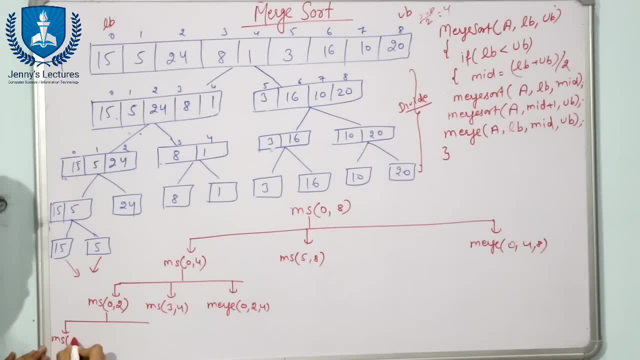 is 1.. Again, call: merge sort: 0 to mid is 1.. Merge sort: Mid is 1, then mid plus 1.. 2 to 2.. Only one element we have now. Now, here we have merging of 0 to 1 and then 2.. Fine, 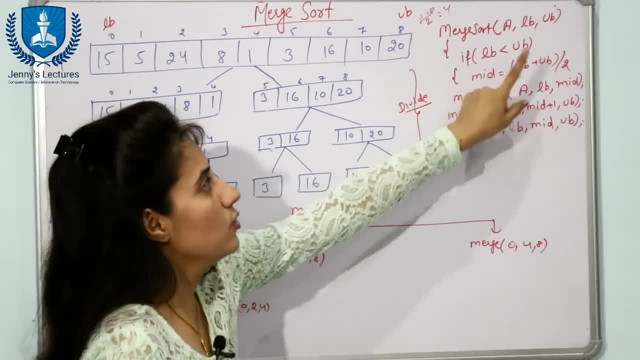 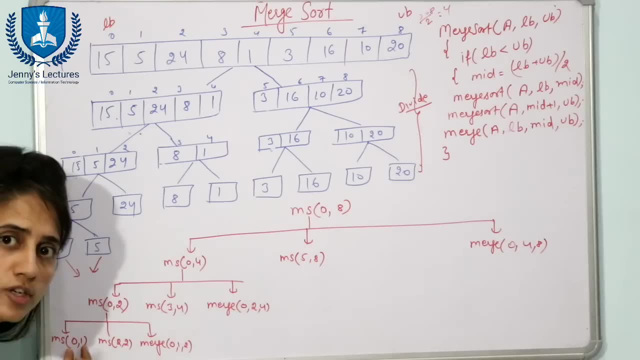 Now, here again: 0 and 1.. 0 is less than 1,. yes, Calculate midpoint. Midpoint is what: 0 plus 1 divided by 2, that is, 1 divided by 2, that is 0.. 0 is midpoint. Fine, So here. 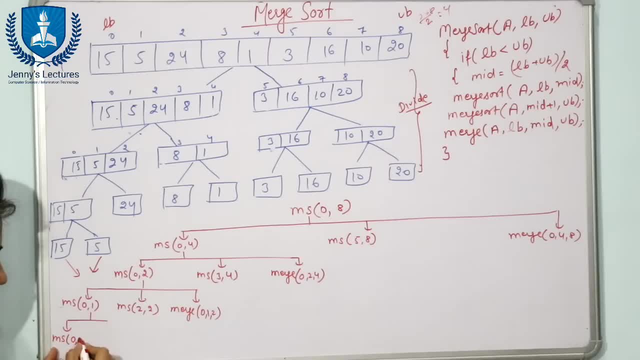 we call merge sort 0 to middle element is 0, because 0 plus 1. That is 1.. 1 divided by 2 is 0. And then again merge sort 1 to 1. And again we are going. 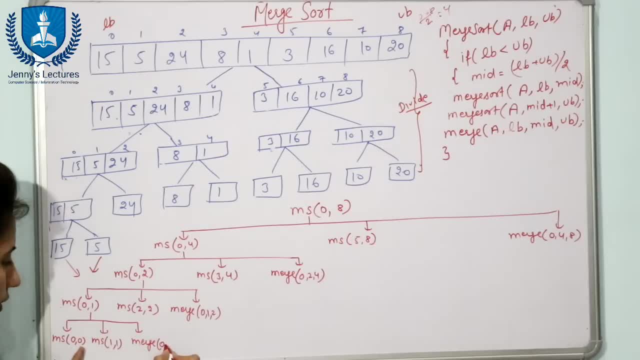 to call merge method on 0.. Middle point is lower, bound is 0,, mid is also 0 and upper bound is 1.. From 0, 0 to 1 to 1.. Fine, Here we have 2, 2.. That is one element. is there? 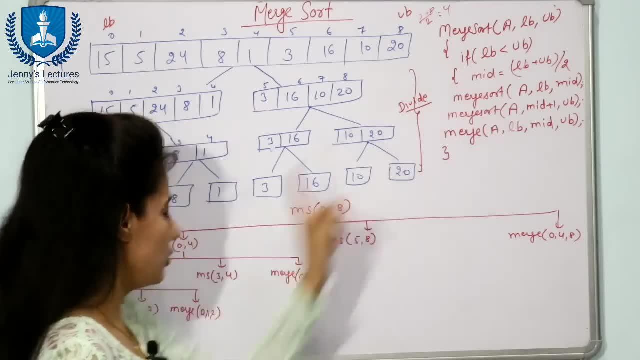 only So we are going to divide this anymore, because lower bound is 2, upper bound is also 2.. 2 is less than 2.. No, this condition is not true, So we are not going to divide this. 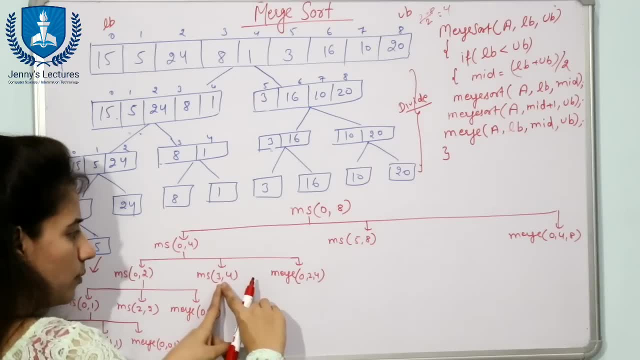 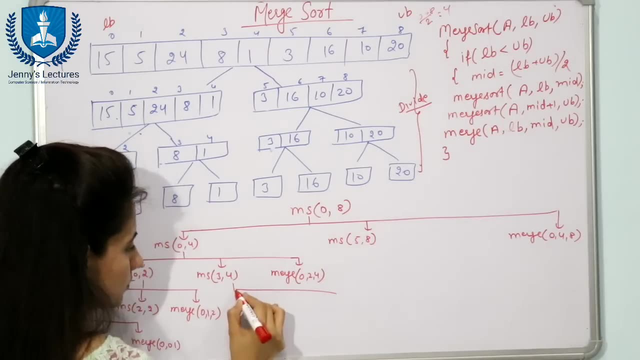 This is merge. Now come to this point. 3 is lower bound, upper bound. 3 is less than 4, yes, Then we are going to divide this into 3 parts, See: 3 is less than 4, yes, Find. 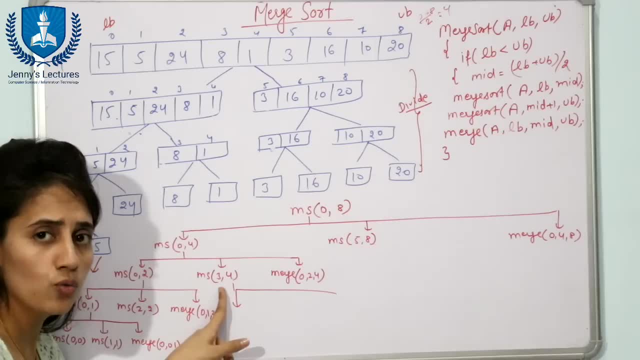 out midpoint: 3 plus 4, that is 7.. 7 divided by 2 is 3, only Fine. So here we are going to call merge. sort 0 to middle. element is 0. 0 is midpoint. That is 0.. 0 is midpoint. 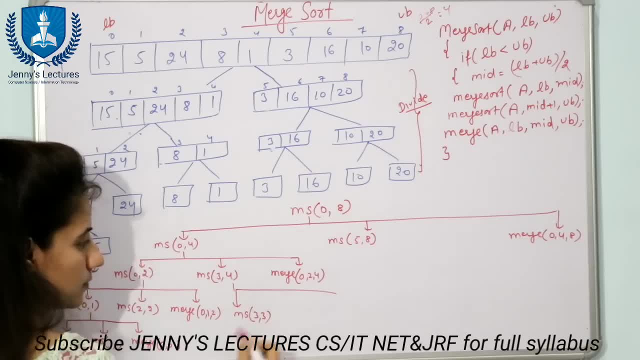 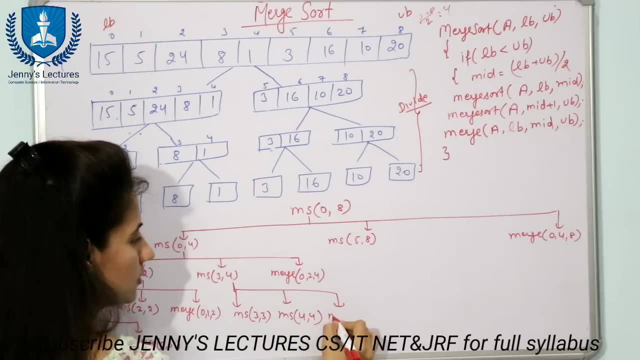 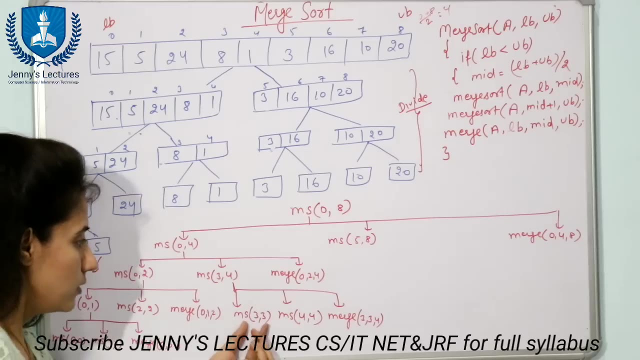 This is merge sort. Lower bound is 3.. Mid is also 3.. Second is merge sort 4 to 4, and this one is merge 3, 3 and 4.. Fine, 3, 3.. Lower bound is 3.. Upper bound is 3.. 3 is less than. 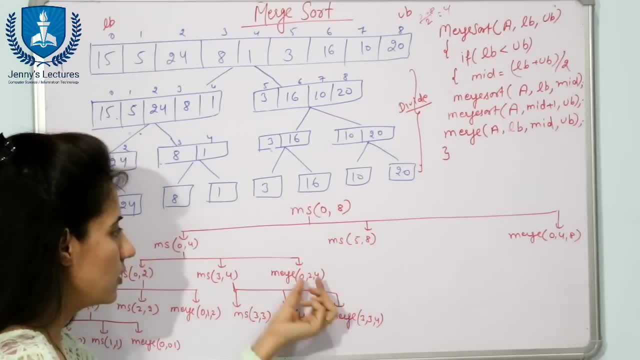 3. No 4 is less than 4.. No, We are not going to divide this Merge this. Then again we have this merge, Then finally this one Merge sort 5 to 8.. 5 is less than 3.. No 4 is less. 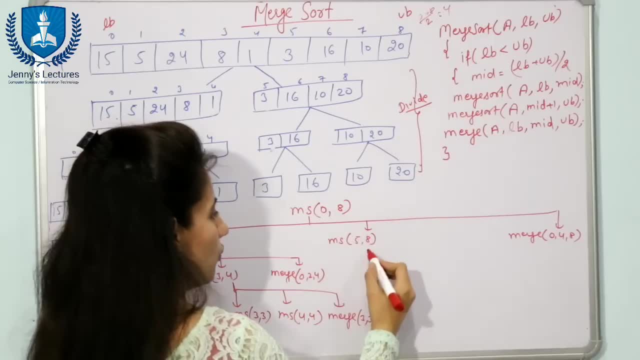 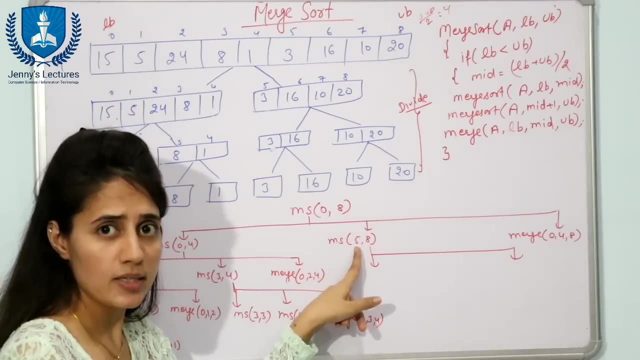 than 8.. Lower bound is less than 8.. Yes, We are going to divide this one. Now see Calculate midpoint: 8 plus 5. That is 13.. 13 divided by 2. That is 6. we have So middle point. 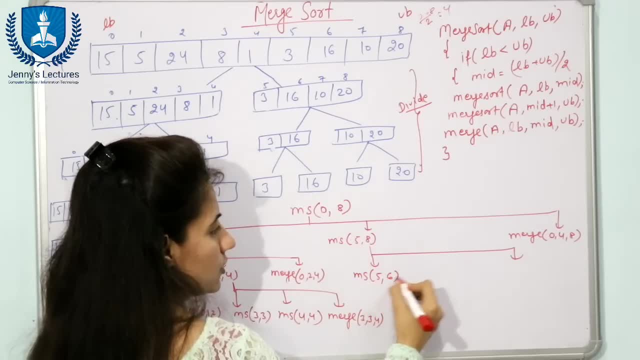 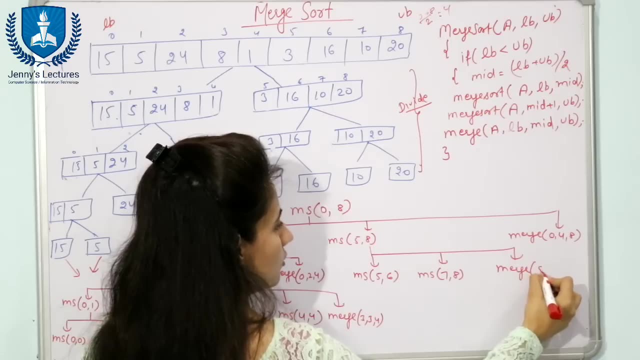 is 6.. Merge sort 5 to 6. Then merge sort 7 to 8. And then we are having merge 5, 6 and 8. Then again come to recursive code to this point. Then again come to recursive code to: 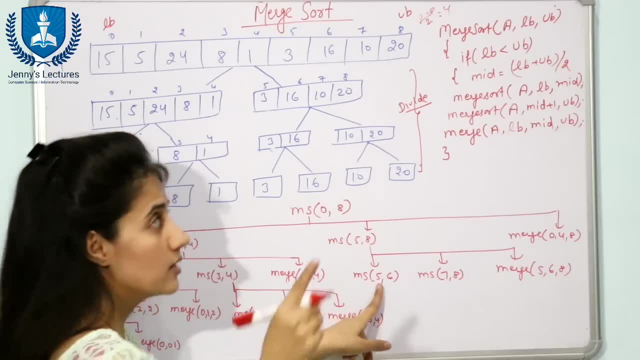 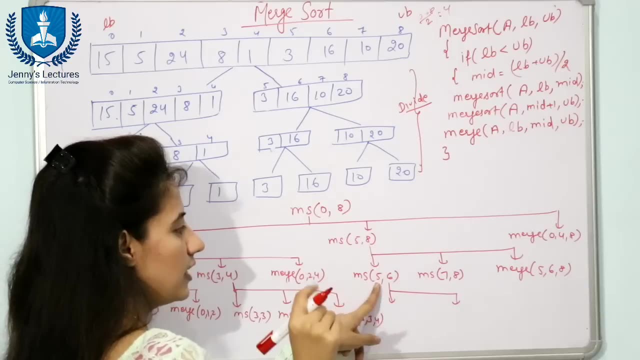 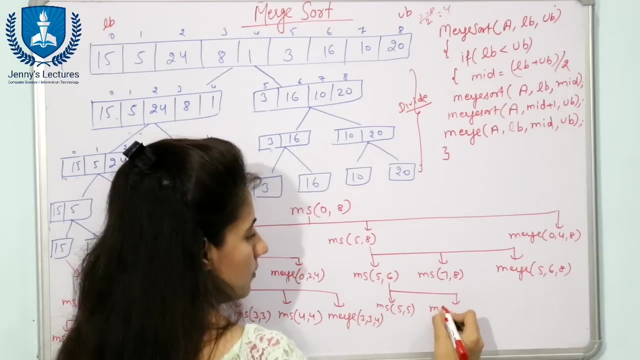 this one, 5 to 6. 5 is less than 6.. Yes, Again, divide this one into 3 parts. Calculate midpoint: 6 plus 5 is 11.. 11 divided by 2 is 5.. So merge sort 5 to 5.. Then merge sort 6 to upper bound. 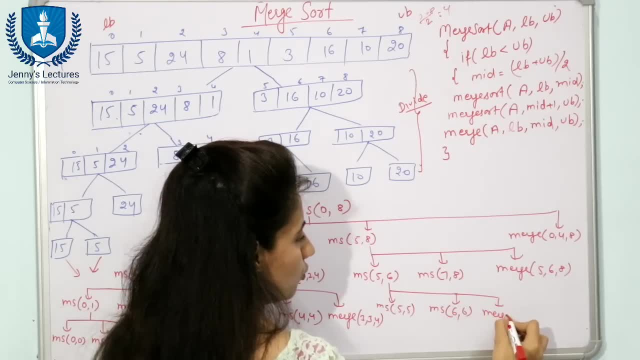 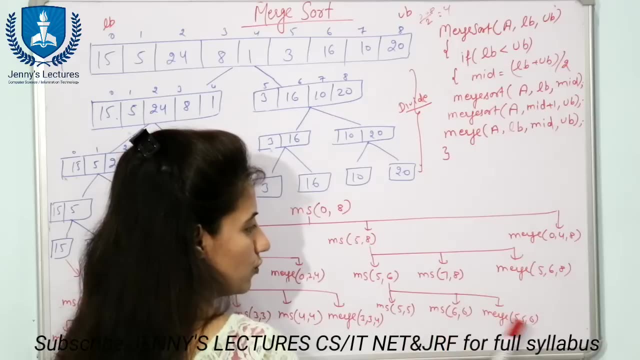 is 6.. Then we are going to call merge 5., Then 5 and then 6.. Fine, Lower bound is 5., Mid is also 5 and upper bound is 6.. Now 7, 8.. 7 is less than this. 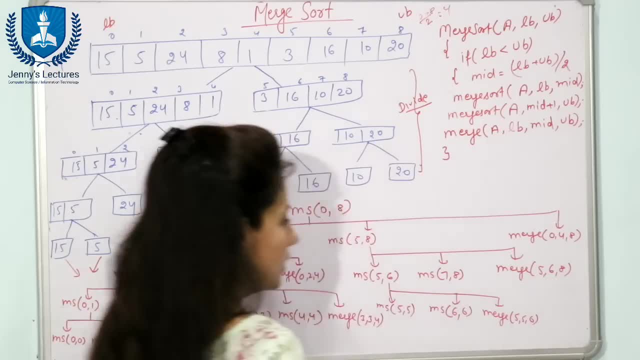 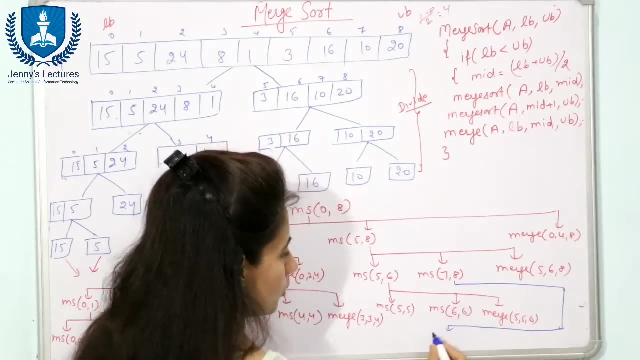 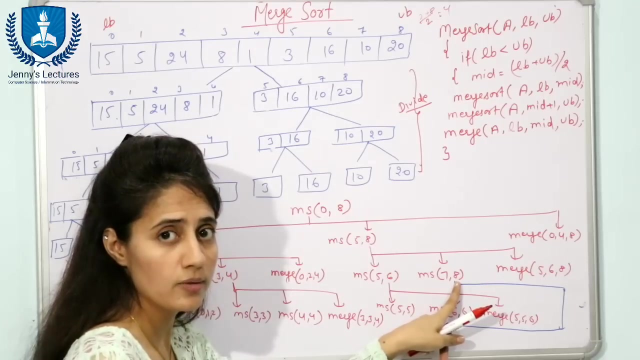 8.. Yes, This condition is true. So again, divide this into 3 parts Now I am going to divide it here only. So now, first is merge sort 7 plus 8.. Calculate: midpoint 7 plus 8 is 15, divided by 2 is 7.. So 7 is midpoint 7 to 7.. Then merge sort 7 to 7.. Then merge. 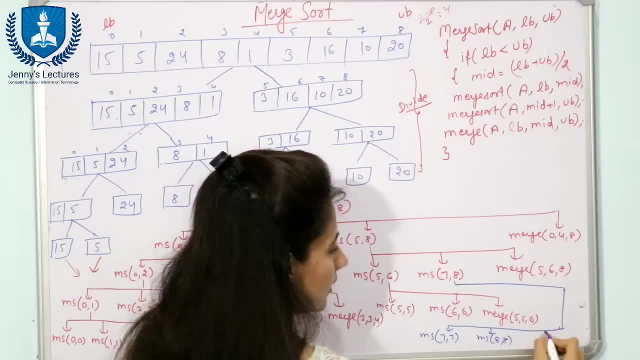 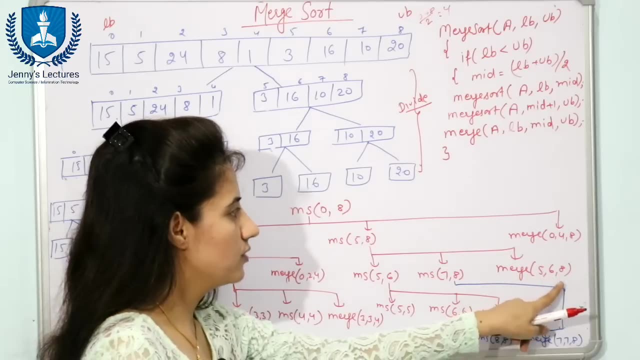 sort mid plus 1.. 8 to 8.. And then we are going to merge 7,, 7 and 8. And finally merge 5,, 6,, 8.. And finally merge 0,, 4 and 8.. So this is the recursive tree. Now how this? 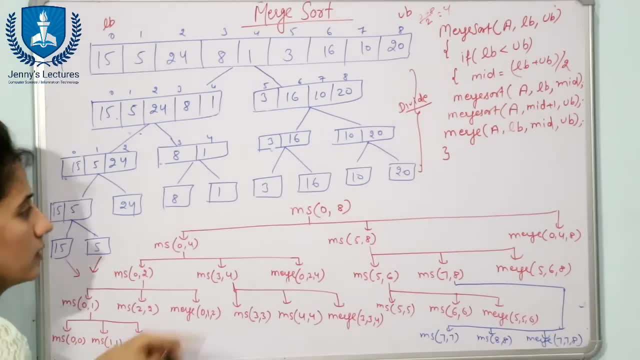 is going to be called, See First of all, merging of 0 to 8.. Here we have. First call would be to this function: 0 to 4.. We are going to first of all call the merge sort 0 to 4.. Again, for sorting of this one. we are supposed to call this one. Again, we are. 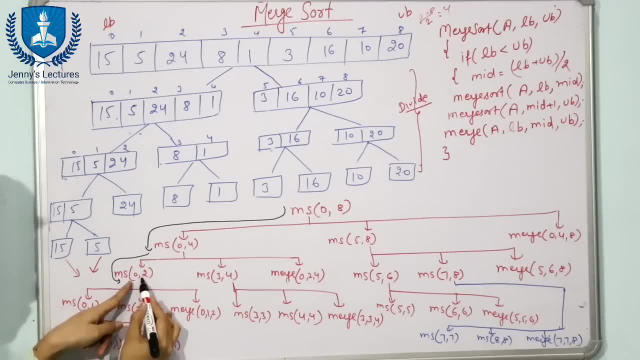 going to call this one 0 to 2.. For sorting of from 0 to 2, we are going to divide this again. So here we go from 0 to 1. only Now for sorting of 0th and 1 element, we are going. 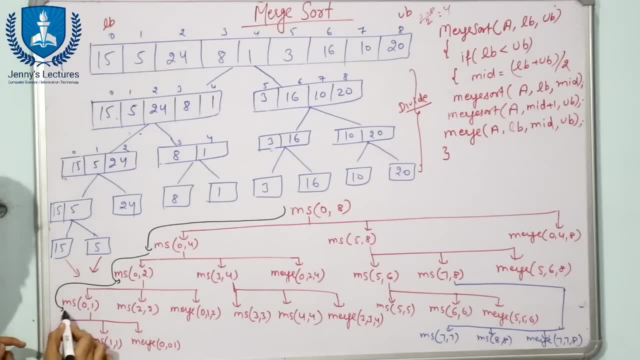 to divide this into 2 halves only. So here we are going to call this one MS 0, 0 and MS 1 and 1.. 0, 0 means we are having only 1 element now 0, 0, that is 15.. Here we have 15 and here 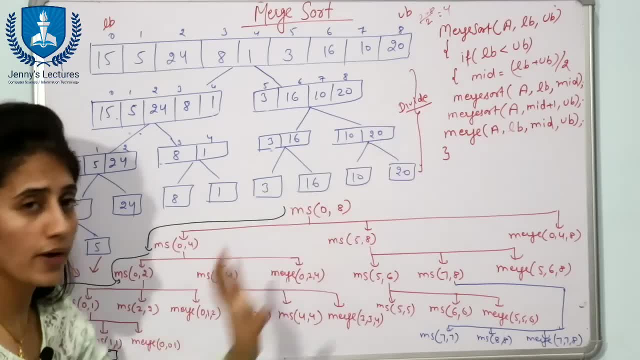 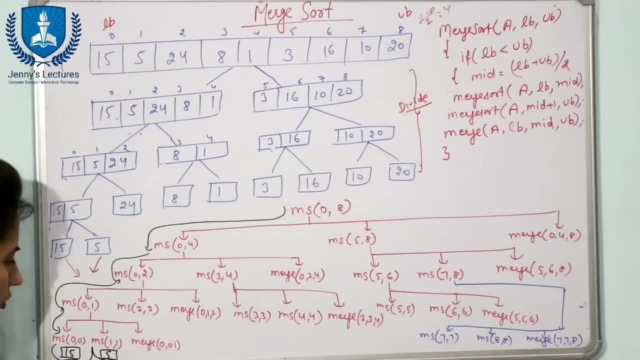 we have only 5 because we cannot further divide it. Fine, So this one is done. This one is done Now. next step is now control would go to this: merge, Now, merging of 0 to 0.. 0 to 0 is 15 and 0, or you can say 0 to 0, then 1 to 1.. 1 to 1 is 5.. 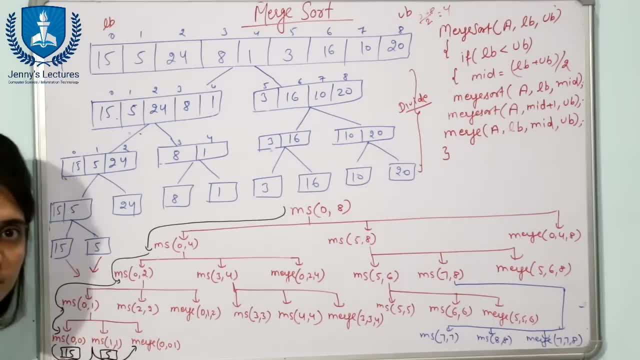 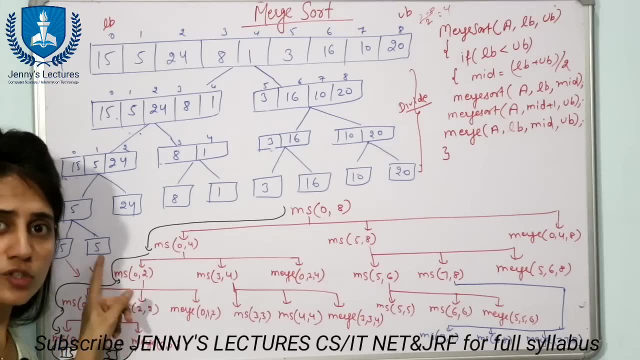 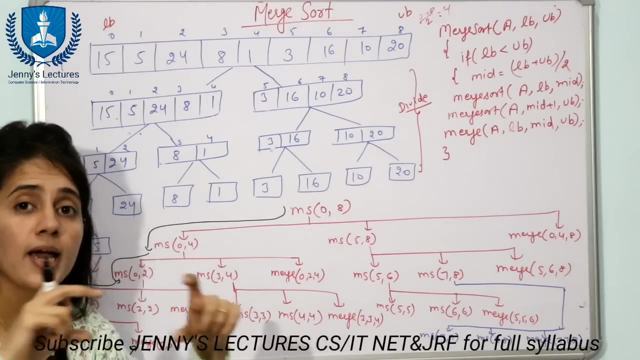 Then you are going to merge this 15 and 5.. Now how this merging is to be done: See 2 sub list are there which are already sorted. You are going to merge those sub list and you are going to produce a new sub list, and that new sub list is also in sorted order. 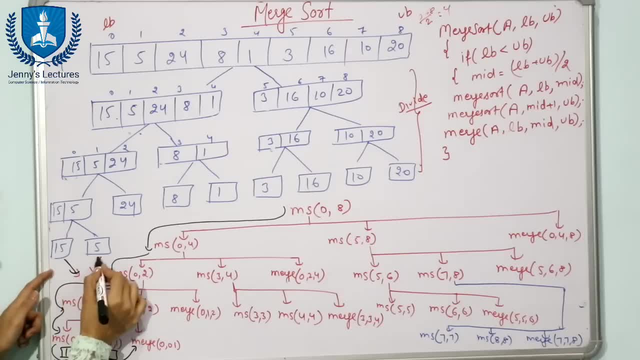 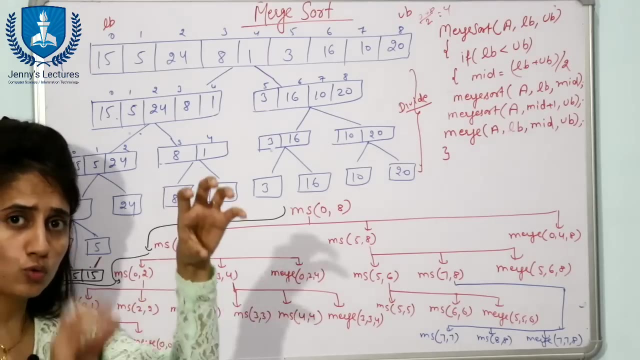 Fine, So after merging of this 15 and 5, the new sub list would be: is 5 and 15? right, how we are going to merge? i am going to explain that processor also, but for now you have to keep in mind that you two sorted sub list are there. you are going to. 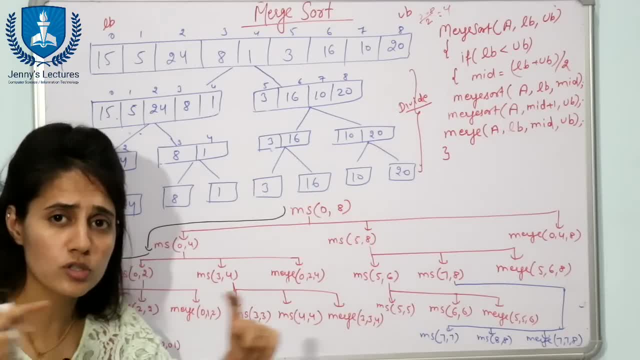 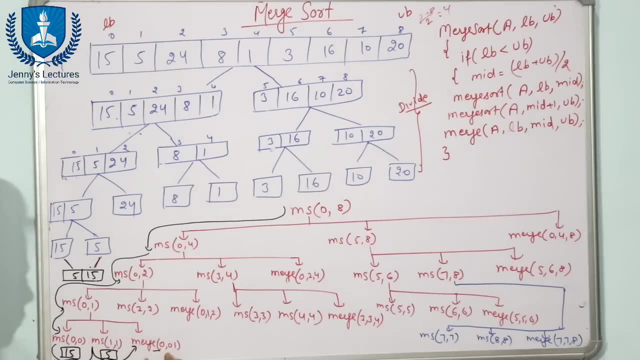 merge those sorted sub list. so the new, new produced sub list would be in sorted order. so this would be 5 and 15. so after merging the list would be 5 and 15, 5 and 15. done now. now the control would go to here only ms 2 and 2, 2 and 2. so this is only one element, is there? 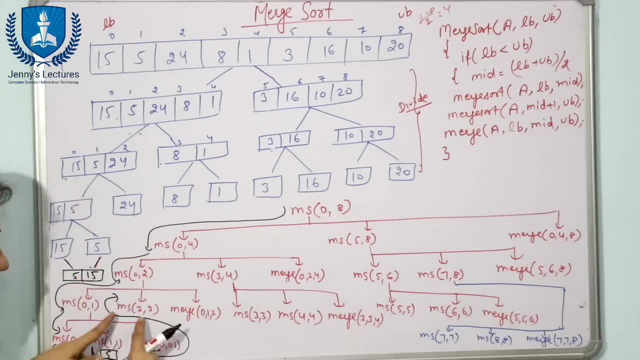 2 and 2. that is 24. fine, now, this one is done. now, 24 is there. 24 is there now. control will go to here: only merge of 0 to 1. 0 to 1. this list and this list is what. 5 and 15, and from 2 to 2, 2 to 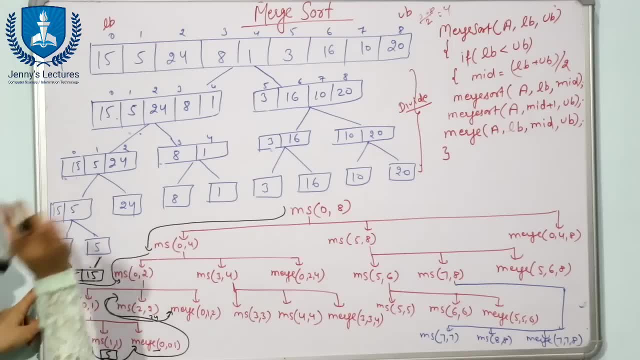 2 is 25.. so now we are going to merge this and this. that is why i am saying you cannot merge this 15 with 8 or 15 with 24, or it's not like that. this 5 and 15 is one list and you are going to merge this. 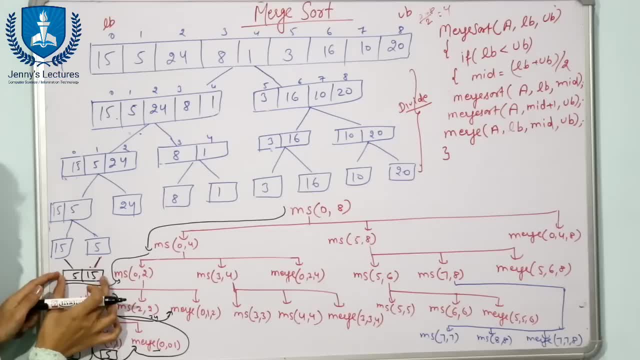 with 8. no, you are going to, you are going to merge these list with its adjacent list only, and when you are going to draw this recursive tree, then you come to know that how we are going to merge these sub list and how you are going to divide these sub list. fine, now this sub list would 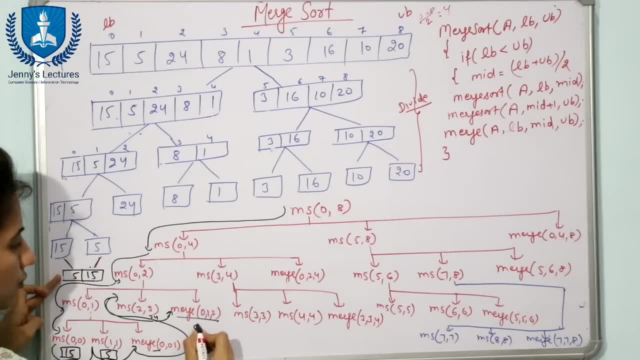 be merged. this and this. now this list would be: 5, 15 and 24. 5, 15 and 24. now, fine, now. now control would go to here, only now. this one is done. 0 to 2. now list. 0 to 2 is what? 5, 15 and 24, the merging. 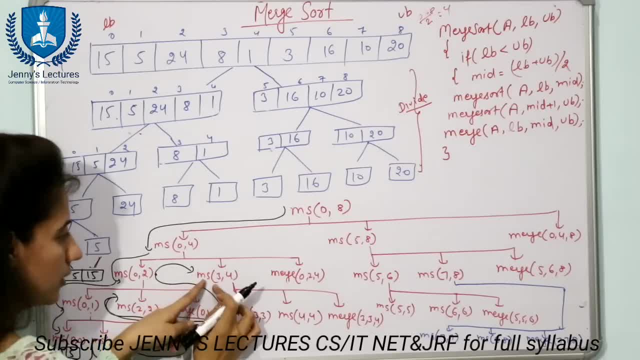 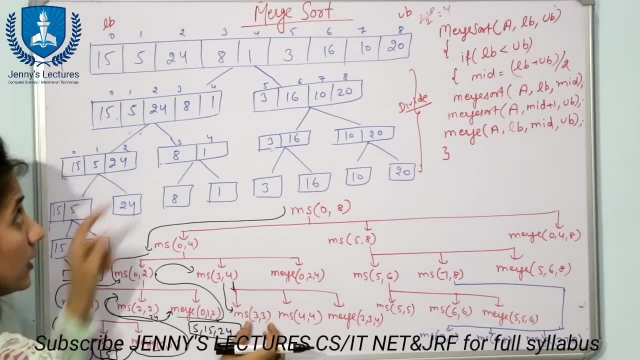 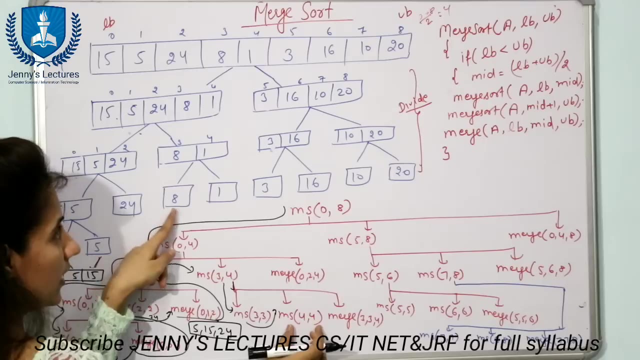 has been done. now control would go to here: only merge sort 3 to 4. now again recursive call. so control would go to 3 to 3. one element is there: 3, 3, that is 8. we are having 8 now. control would go to here: 4 and 4. one element is there that is. 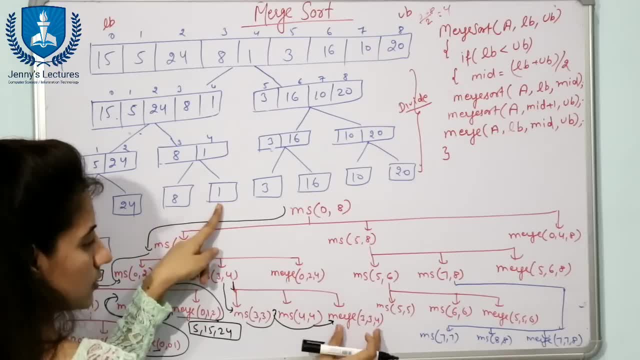 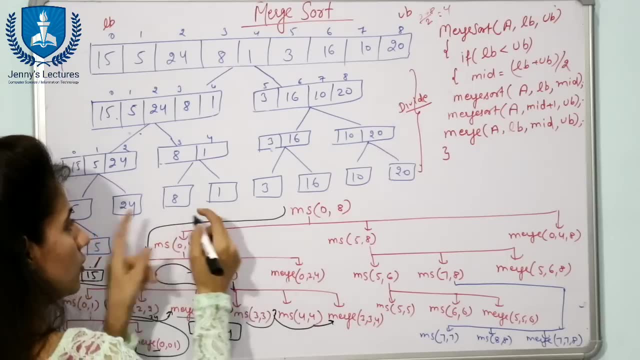 1, only now. control would go to this merge. we are going to merge 3 to 3. 3 to 3 means 8, and then 4 to 4, that is 1. so we are going to merge these two and the result would be: 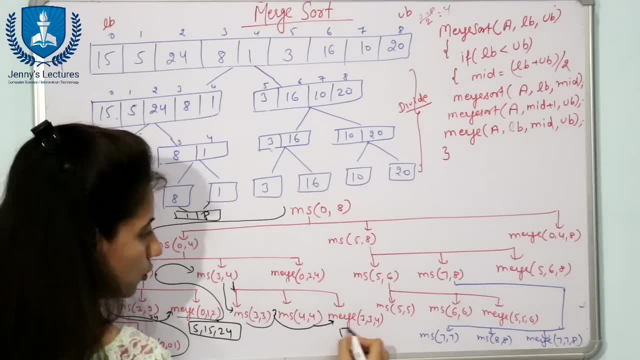 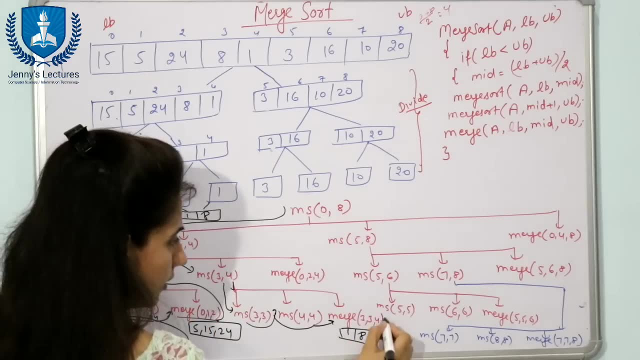 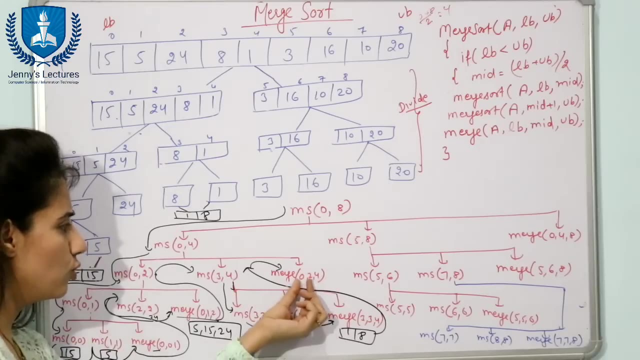 1 and 8. fine, so here we go to what: 1 and 8 after merging. i am going to discuss this merging method also now. control would go to here, only now. this one is done. now control would go to this merge: now we are going to merge from 0 to 2. 0 to 2, this one and 0 to 2. the list is this one we have. 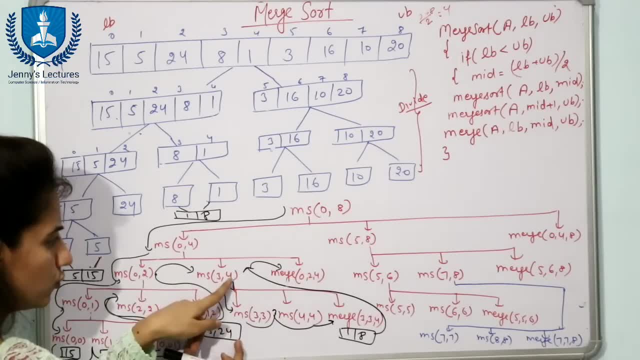 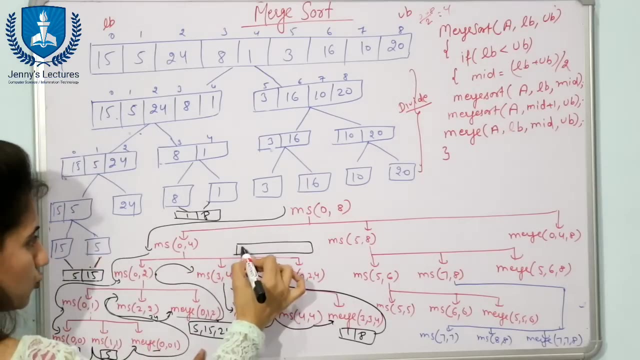 got this list fine, and from 3 to 4, 3 to 4, the list is 1 and 8. now we are going to merge this 5, 15, 20, 4 with 1 and 8. fine, and after merging of this 2, now the list would be this: 1, 5, 8, 15 and 24 at this. 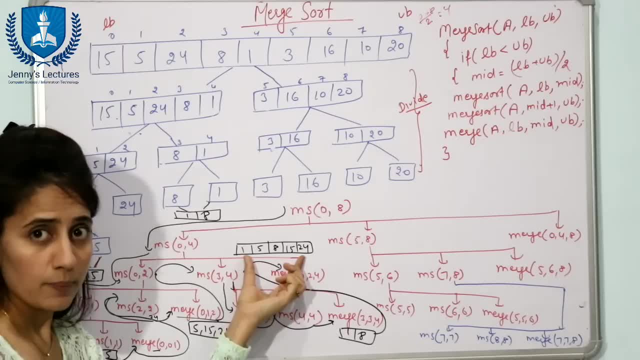 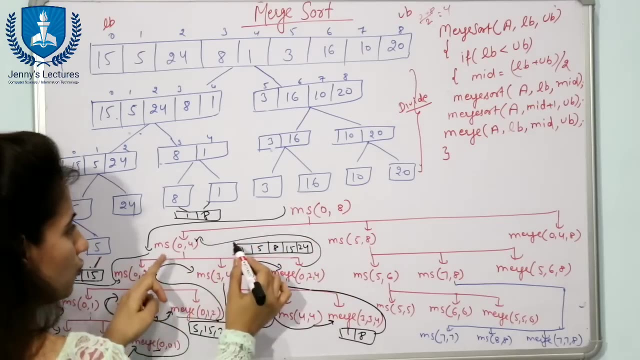 step. you are going to find out this result because when you are to sort, when you are merging two sorted sub list, then result result would also be a sorted list. fine, now, now this one is done. now, again we have done from 0 to 4. now control would go to from 5 to 8. now again this same. 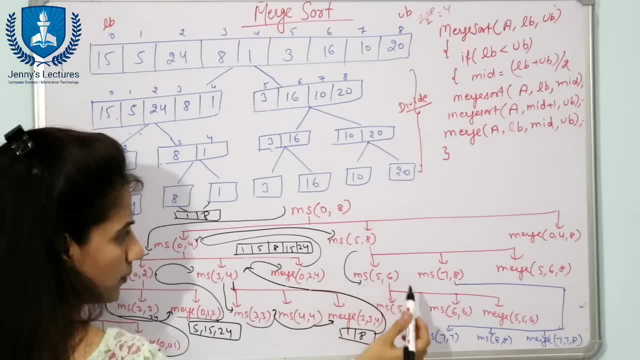 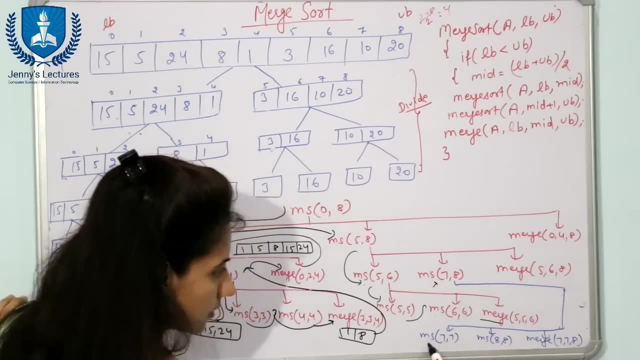 processor would be there, the control would go. recursive call is there. so from 5 to 6, then from 5 to 5, then here 6 to 6, then merging would be done. then again back to 7 to 8, then this one, this one. 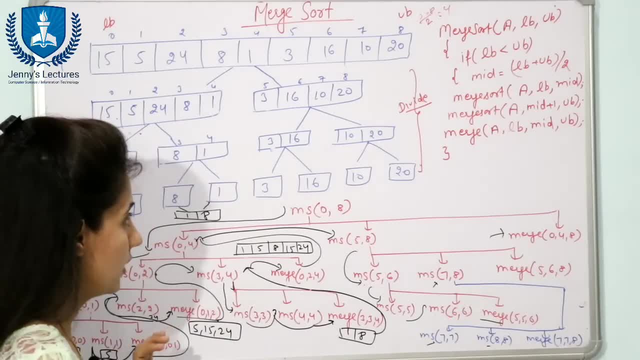 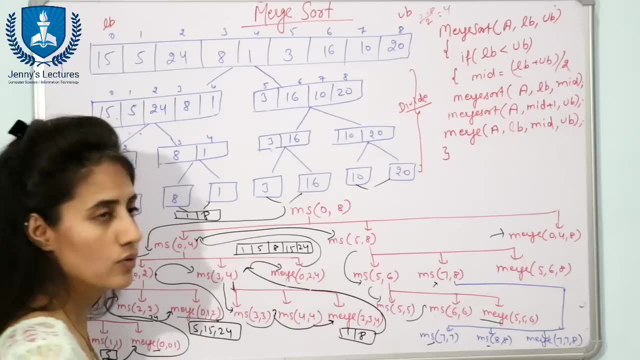 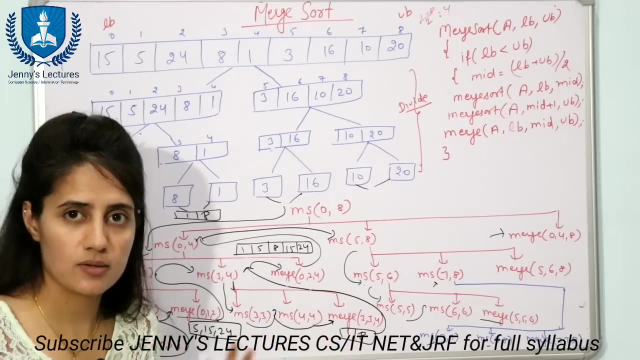 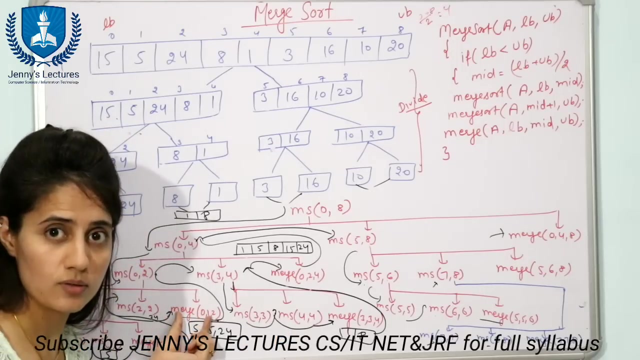 this one, and then, finally, merging of these list. fine, so here, merging of these two, then merging of these two- fine, and ultimately you will get one complete sorted list. fine, now I am going to discuss with you how this merge function is going to be executed. now check, we are going. 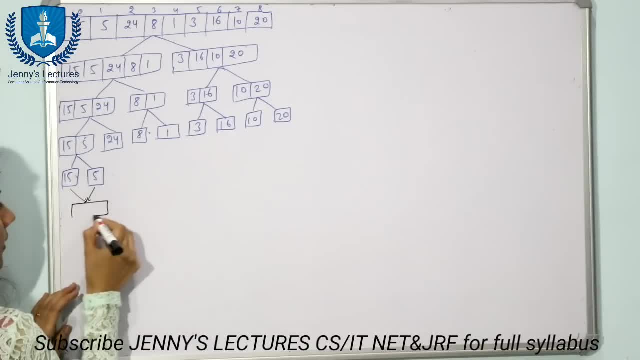 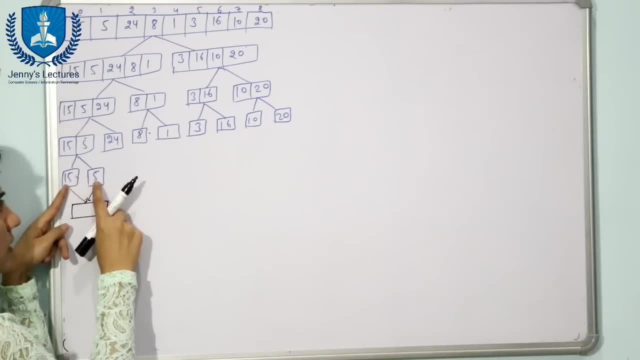 to merge first of all these two and how merging would be done to sub lister. there we are going to compare the first element of these sub list, 15 and 5, which one is less, five is less. So we are going to put 5 first of all, then we will put what 15.. 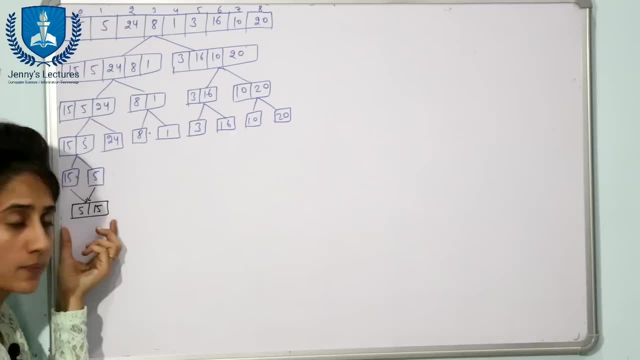 So this is the new produced sub list, sorted sub list. fine, Now this would be: this would be merged with this 24, this 24.. Now the new sub list would be 5, 15, in one sub list. we have 5 and 15, in one we have. 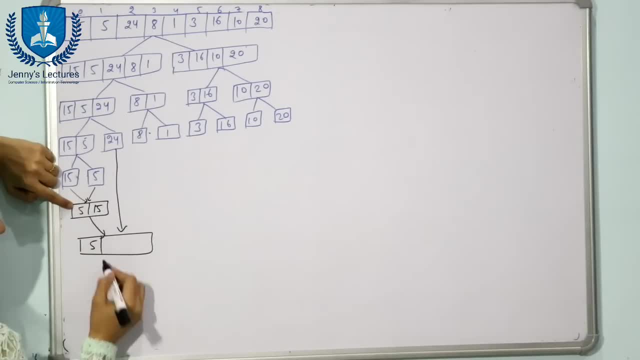 24,. now compare 5 with 24, which one is less 5, so we will put 5 here, then 15 with 24,. 15 is less, then we are going to put 24,. this is the new sub list now. 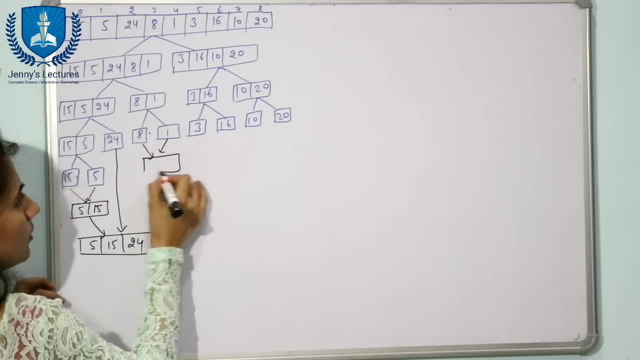 Now 8 with this 1, and the new sub list would be 1 and 8.. Now this with this 1 and 8, so finally, the new sorted sub list would be: see: compare 5 with this 1, which one is less 1, 1, then here we have 8, here we have 5, 5 with this. 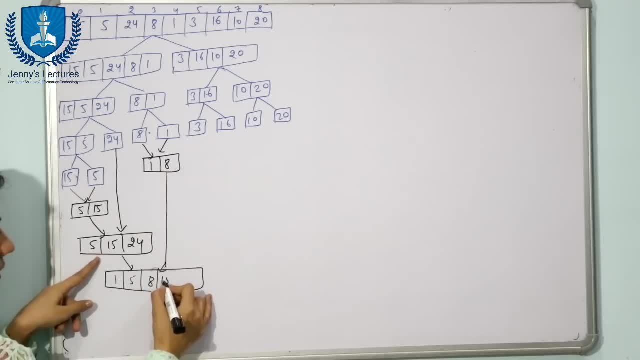 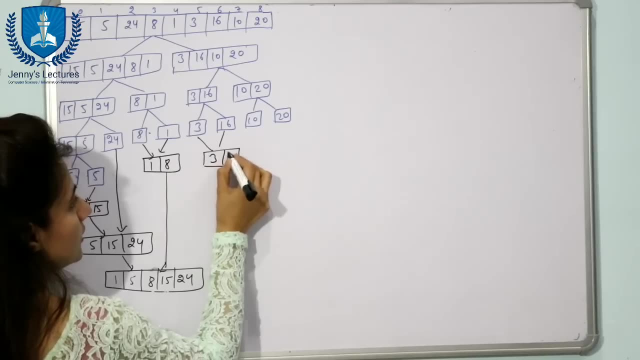 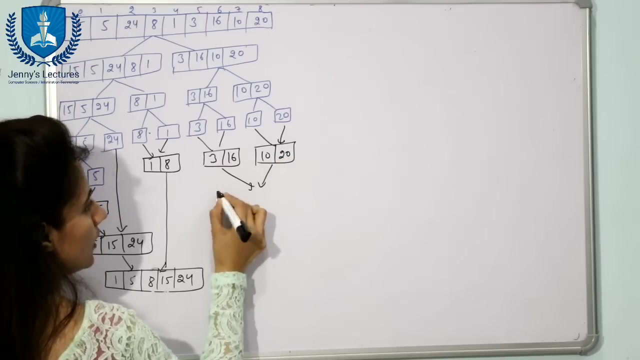 8,, 5.. Then 8,, then 15,, then we have 24,. fine Same here. we have 3 and 16, here, after merging, we will get 10 and 20,. after merging of these two, what you will get: 3,, 10,, 16 and then 20.. 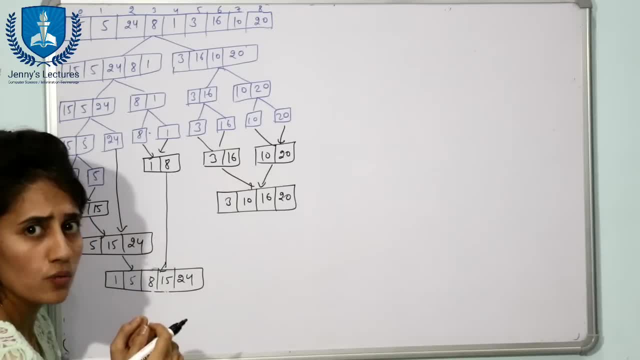 Now we have two halves: one is this one and one is this one. Now, finally, you are going to merge these two And ultimately you will get what one list. that would be sorted fine, And then we will stop what merging fine. 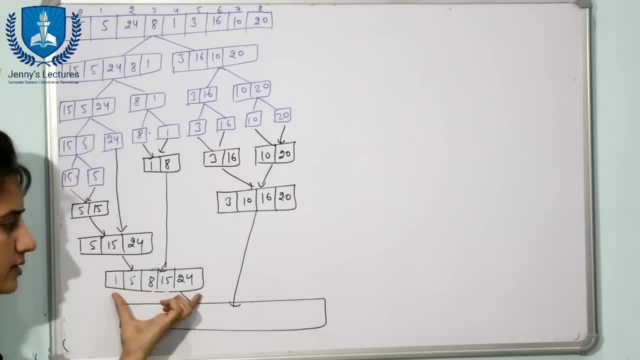 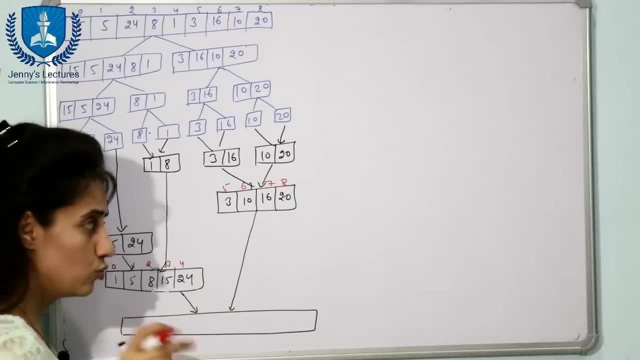 Now see: now this sub list is there, and this sub list is there Now how merging is to be done? let us see. So now we are having two pointers. one is suppose I pointer that would be pointed to. 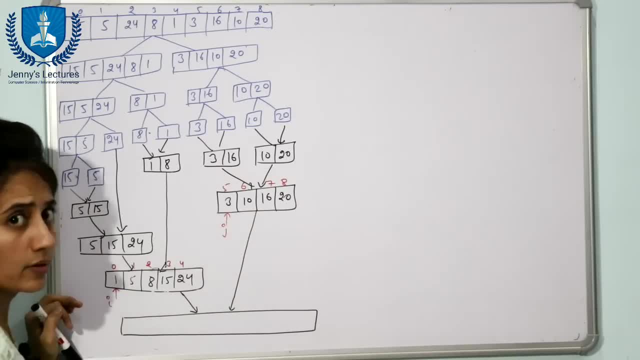 this lower bound. one is this: J pointer: Okay, One is this and one is this one. maybe you can say: this is left and this is right sub list. Another list is there. we are going to produce another sub list. sorted sub list. fine. 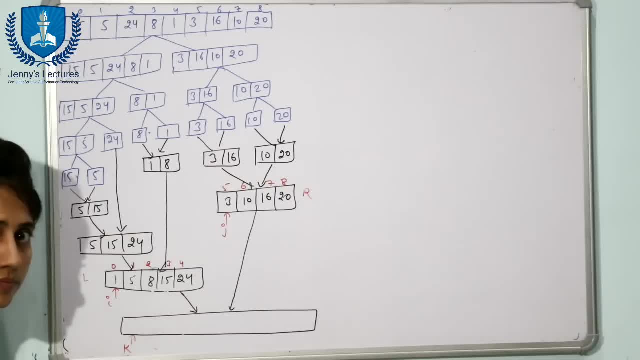 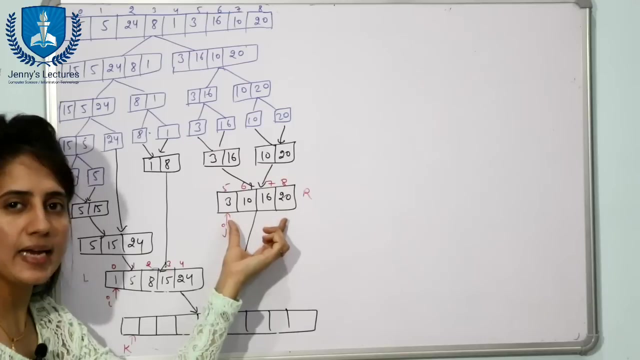 Another pointer is there that is K, which is at the starting of this sub list. fine, And how many elements would be there in this sub list total of this and this one? Let us suppose here we are having M element, here we are having N element. 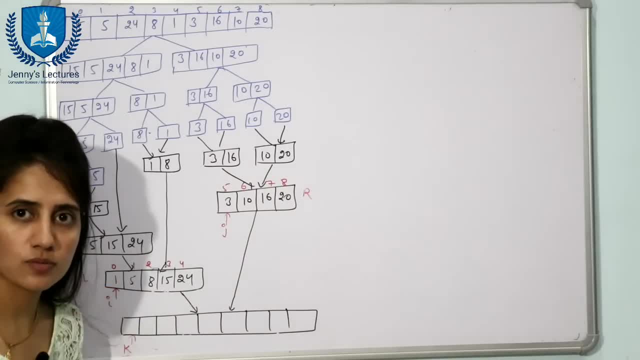 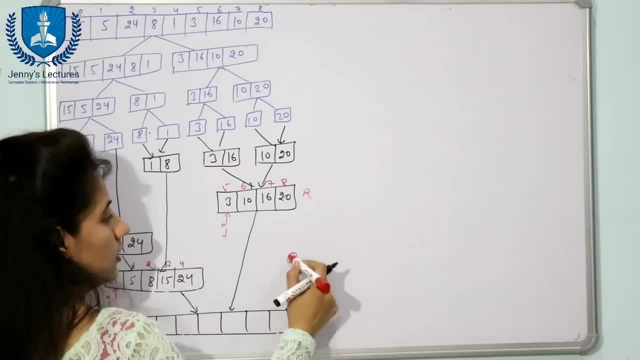 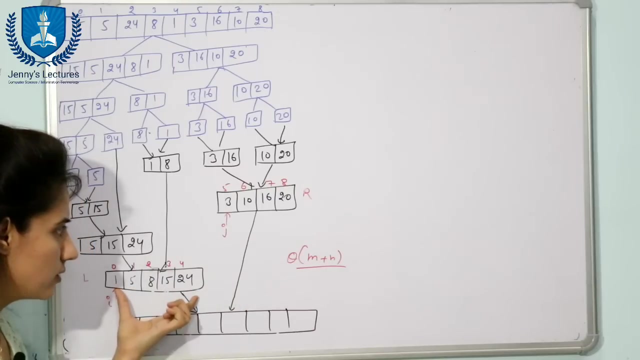 So total would be what M plus N elements. fine, So this merging, this merging function, the time complexity for this merging function would be what Theta M plus N. M is number of elements in one sorted sub list. N is number of elements in another sorted. 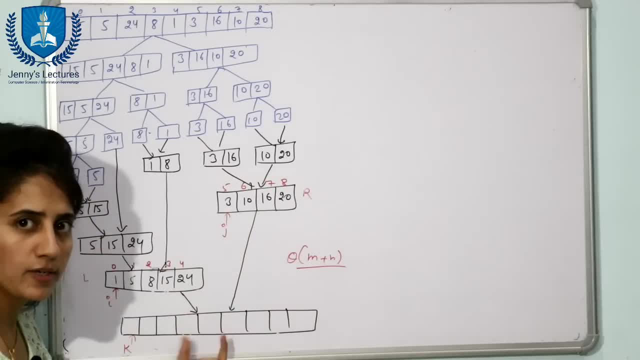 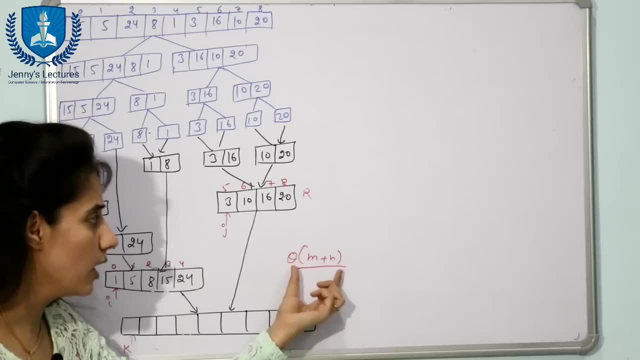 sub list. When you are going to add these elements into this one, then how many elements would be there in this K in this sub list? M plus N. So time complexity for this merge function would be Theta M plus N. fine. 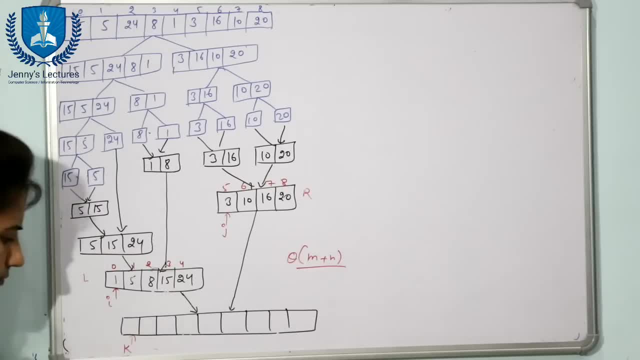 Now how merging is to be done. First step is we are going to compare now first element of this with this. Or you can say: suppose name is L, this name is R. So now we are going to compare L of I with R of J. 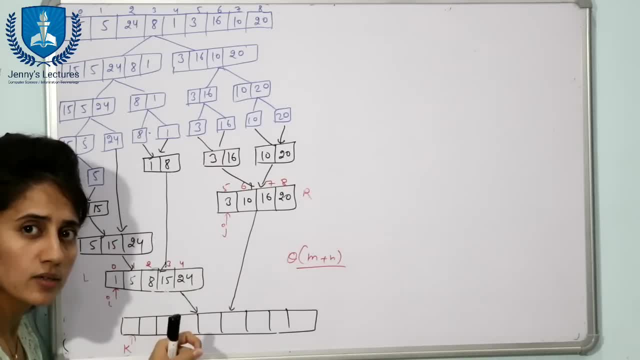 And which element, which element which is less. we are going to put that element into this sub list. fine, So now we are going to compare L of I with R of J, So 1 and 3, which one is less? 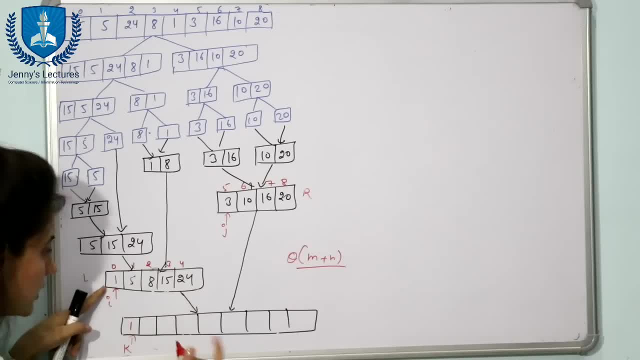 1. So we are going to put 1 here. Next step is we are going to increment this K. Now K is at this place And we have placed 1 here, So now we are going to increment this. I also. 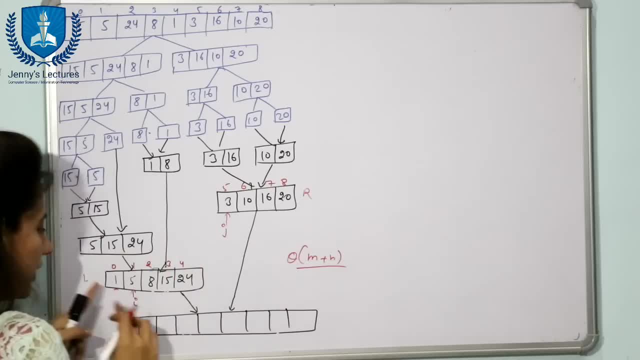 Now I is at this place. Now again, compare L of I with R of J, 5 and 3. Which one is less 3.. So we are, we are going to put 3 here Again. we are increment this. 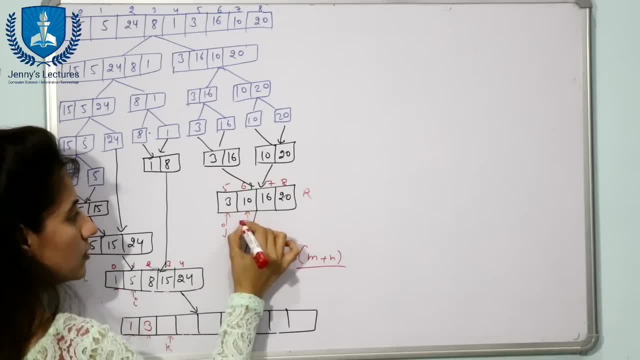 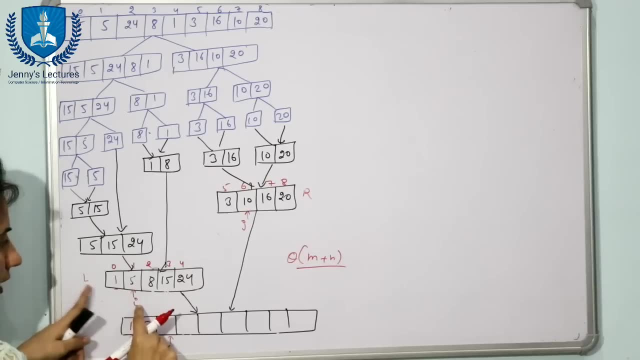 K and we are incrementing now this J Because we have put this 3 here only. fine, Now again, compare L of I, 5 with R of J. that is 10.. 5 is less than 10.. So we are going to put 5 here only. 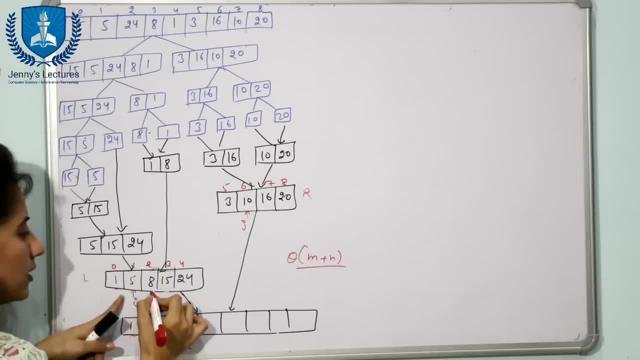 Increment K. K is now at this place And increment. I now Now again compare 8 with this 10. 8 is less than 10. So we are going to increment this, So we are going to put 8 in this new sub-list. 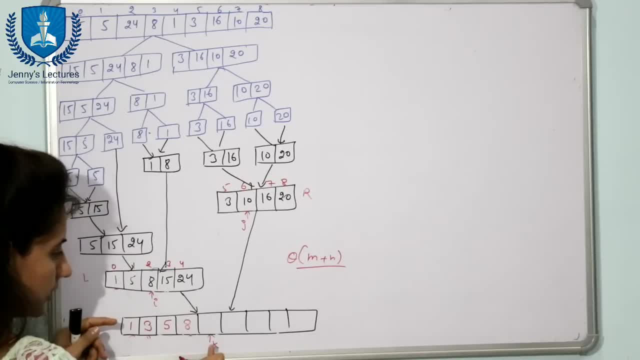 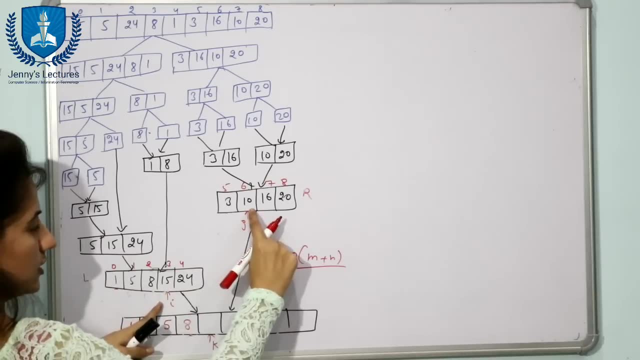 Now increment this K- Now K is at this place- And increment also. I Fine, Now again, compare 15 with this 10. Which one is less 10.? So we are going to put 10 in this sub-list. 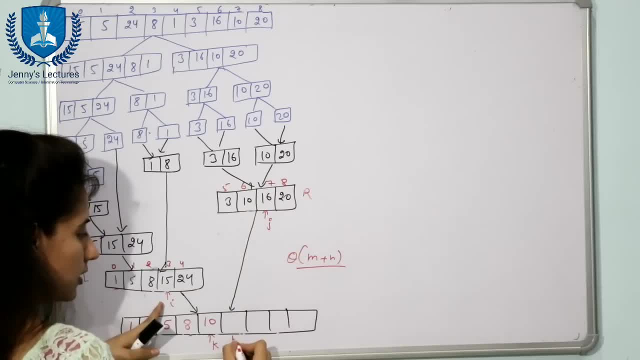 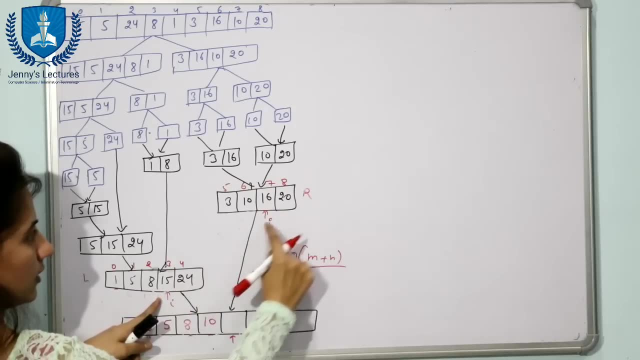 And increment this J- now J is at this place. And increment this K- now K is here. now Again, compare 15 with this: 16. I is It is here and J is here. only 15 is less than 16.. 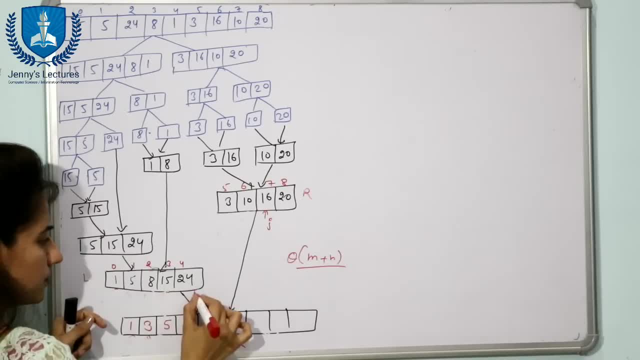 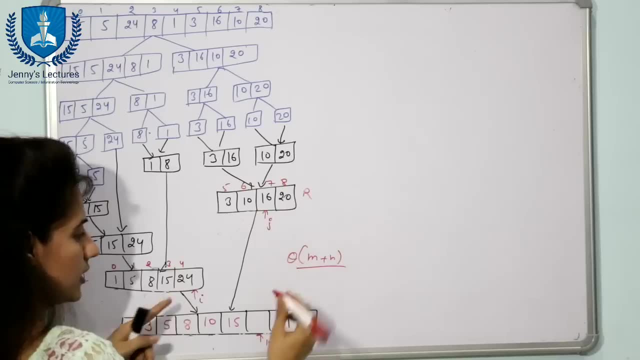 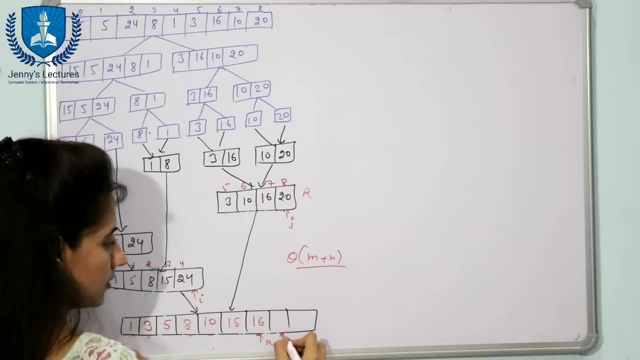 So we are going to put 15 here. So now increment I And increment K, 24 and 16.. Which one is less 16.. So we are going to put 16 here. Now increment this J and increment this K. 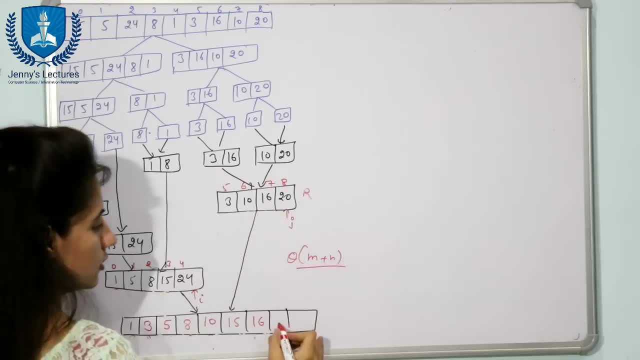 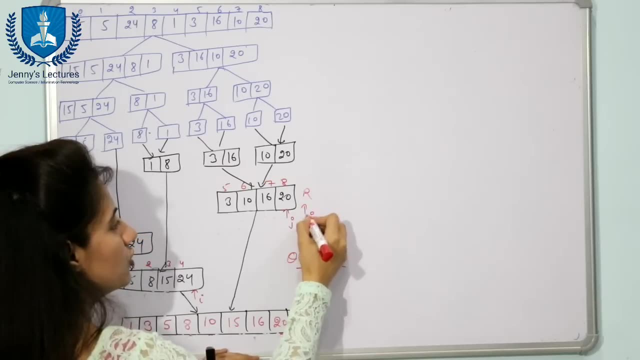 Fine, Now 24 and 20.. Which one is less 20.. So we are going to put 20 at this place. Now increment this K and if you increment this J, now J is greater than this upper bound. 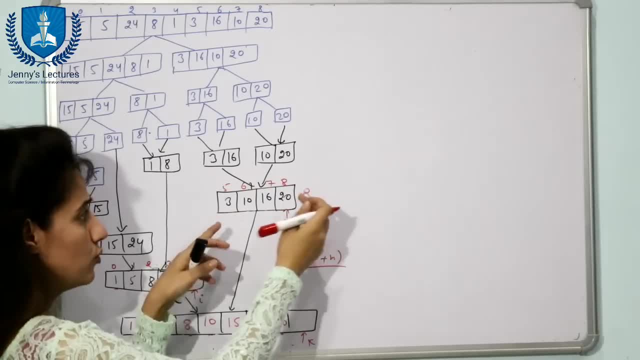 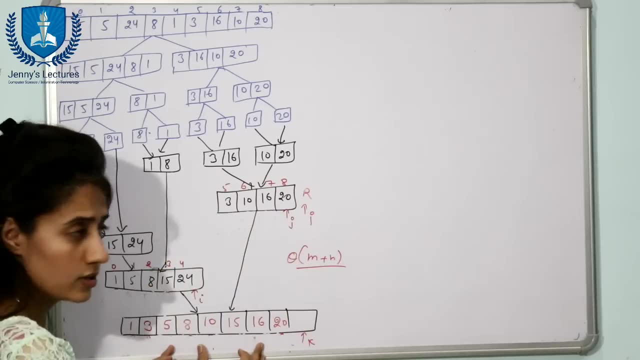 Fine, It means this list is now exhausted. Means: you have put: you have already put this element, all the element of this sub-list, into the new list sorted sub-list. Fine, So this is now done. Now what you have to do? 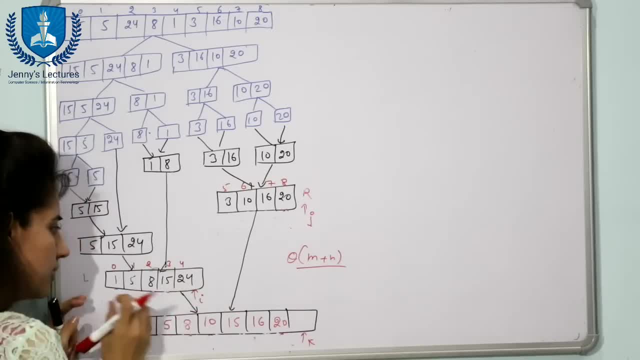 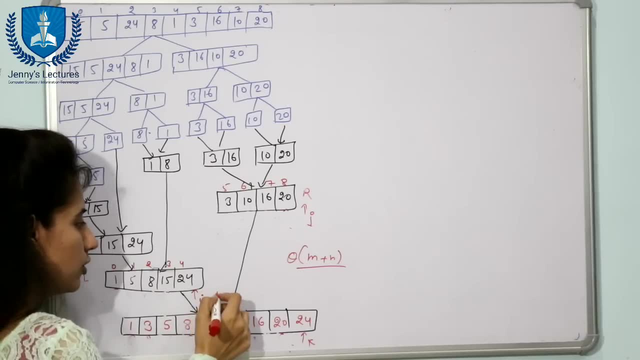 Now, one element of this sub-list is remaining. Now you simply simply put this element, One element, into this sub-list 24.. Fine, And we increment I. so increment is also now greater than this element, So this one is also done. 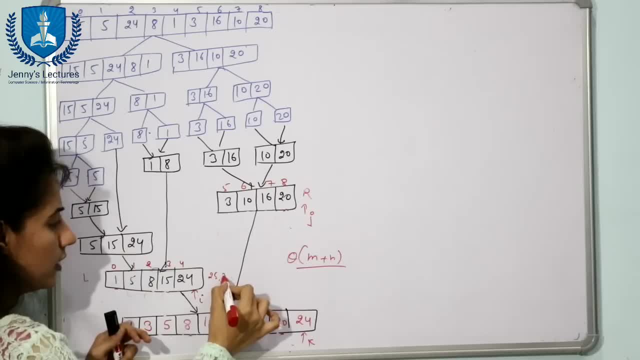 Now, if suppose here, 25 is also there, 30 is also there. Now, what you will do Now? see, this list is done now. So you simply put all the remaining elements of this sub-list into this one: 24,, 25 and 30, like this: 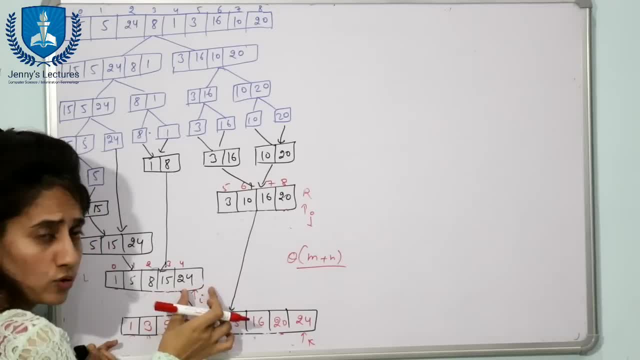 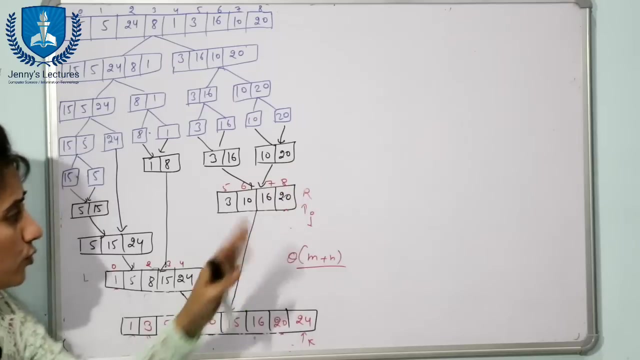 Fine, Here, in this case, only one element left over, so we simply put 24 here only. so this is now the sorted list. fine, after merging of these sublist. so this is, this is how the merging is to be done. fine, so now, if you write down the code for this merging technique, then how you will write. 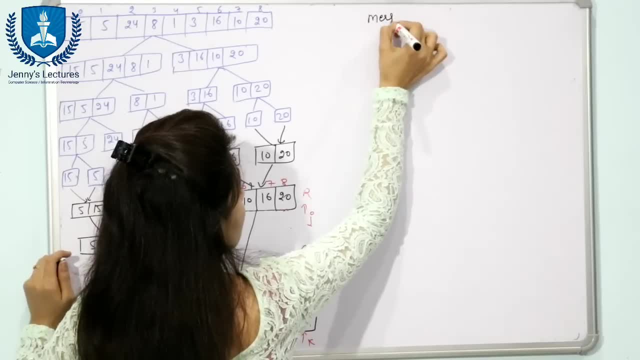 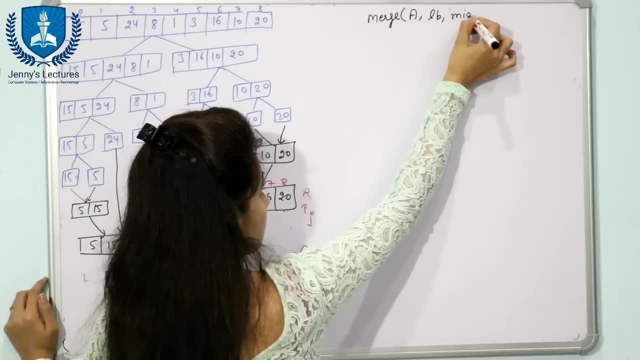 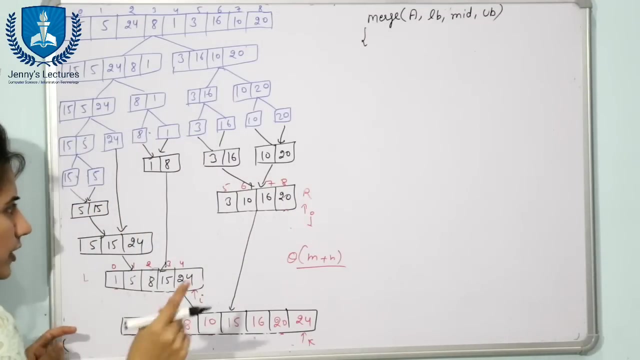 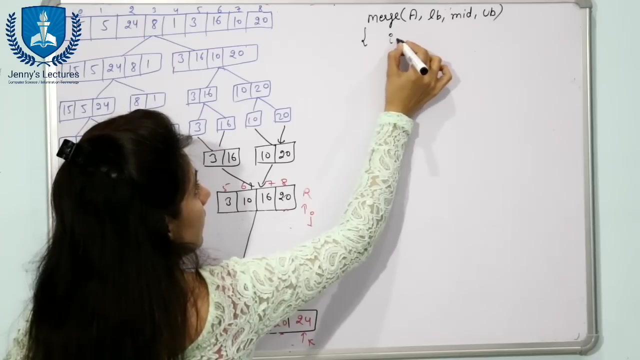 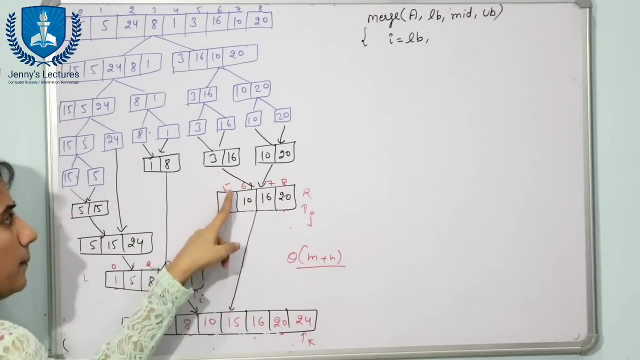 see, we are having function merge. merge, fine, array. we are going to pass lower bound, then we are going to pass mid and then upper bound. fine, now next is see, we are going to take i, j and k, three variables, and i is equal to from lower bound and j would be, j would be from mid plus one because, see here, 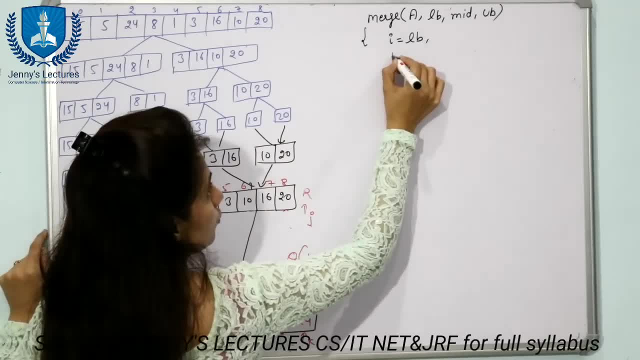 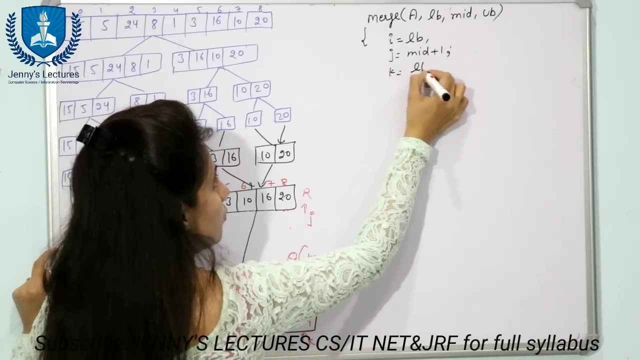 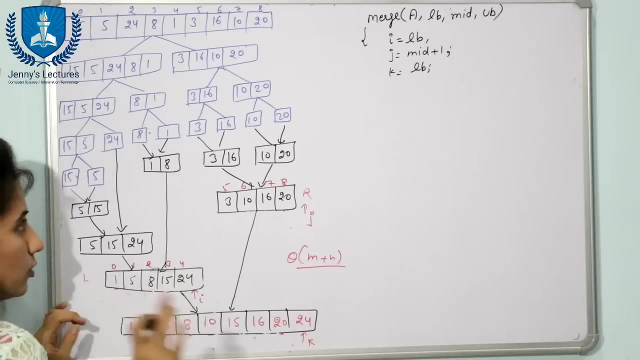 mid is what. four, so j is from here, five, so j would be from mid. plus one and k would be, is equal to: from lower bound, only from zero, only now. next, what you are going to check is: you are going to write down a loop. while this i is less than equal to mid, this i is less than equal to mid and plus this j value is. 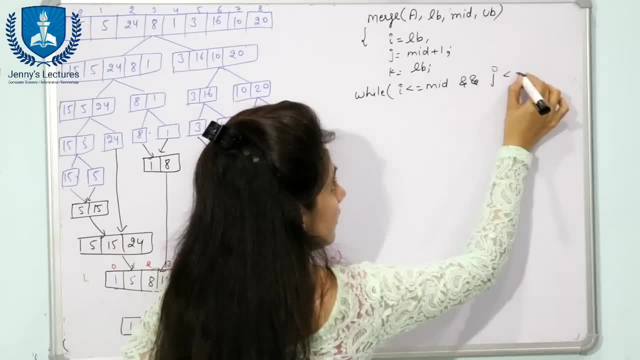 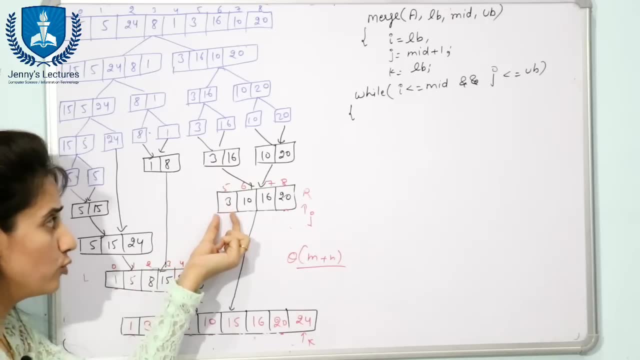 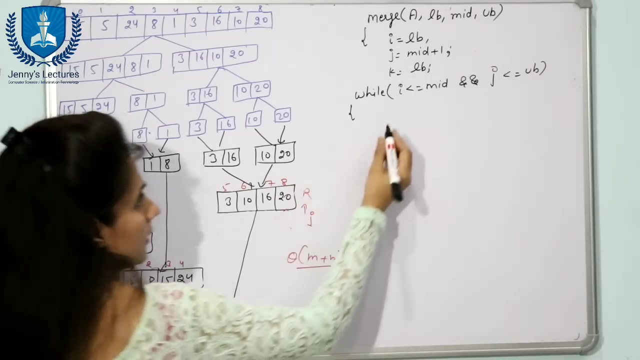 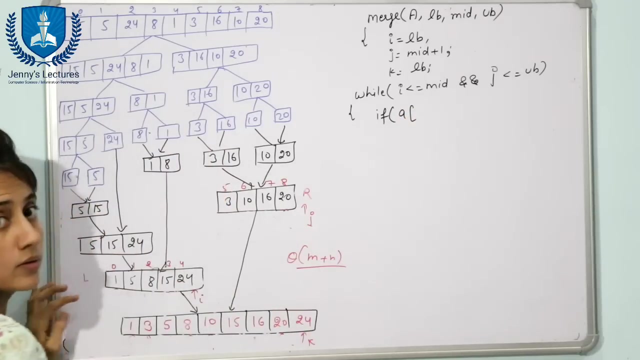 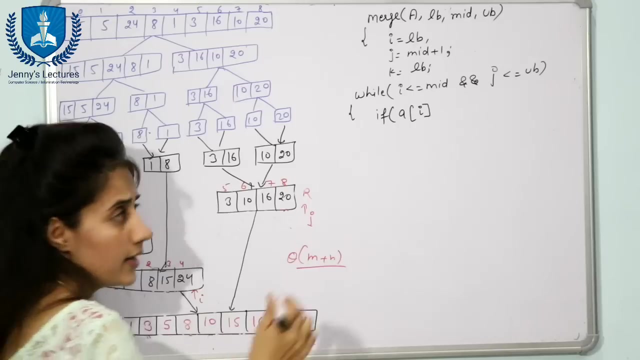 less than equal to upper bound than equal to upper bound. In that case only, you are going to compare these elements and you are going to put the element which is lesser into this new array. Fine, So now you compare. If A of I see name of this array- is A, A of I is less than than equal to A. 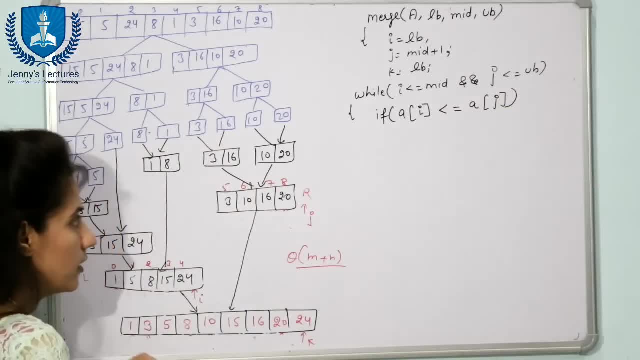 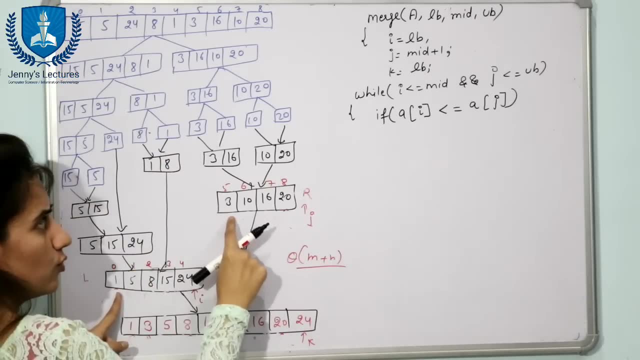 of J. Fine, Because the array is this array name is A only, So A of I is less than equal to this A of J. Then what you will put? You will put this A of I into this array, So we are going to. 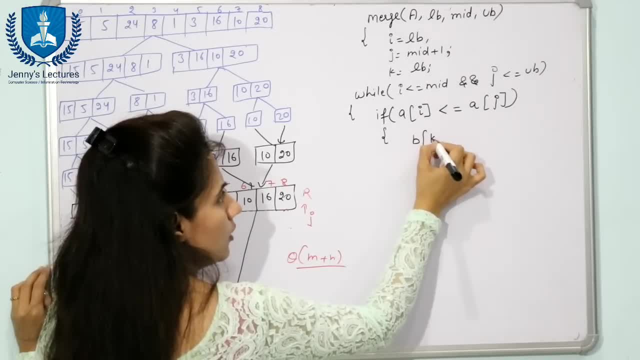 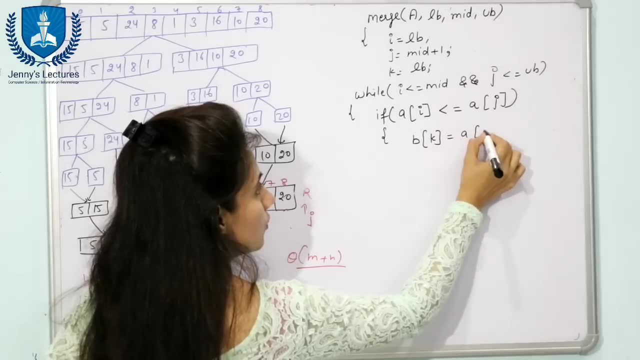 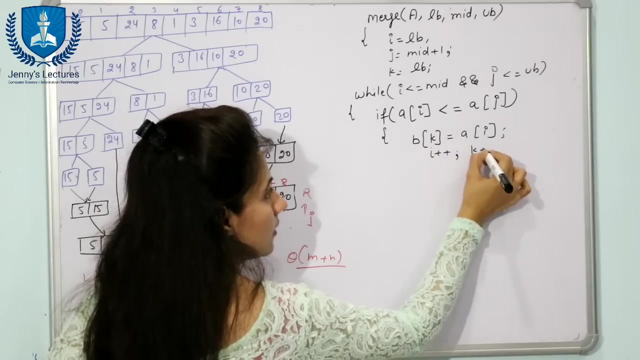 take another array that is name is B, So B of K. See, we have taken one variable, K, So B of K is equal to A of I. Fine, And next what we have done: I++ and K++. Right, Else. 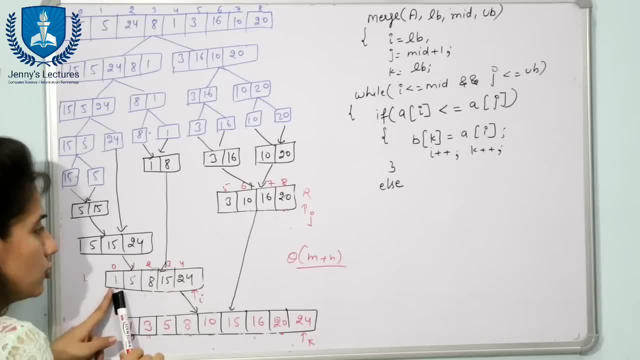 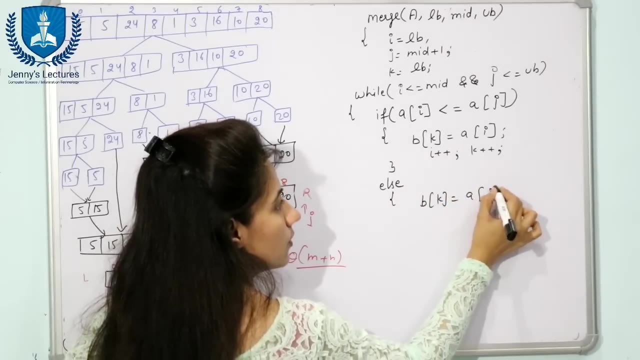 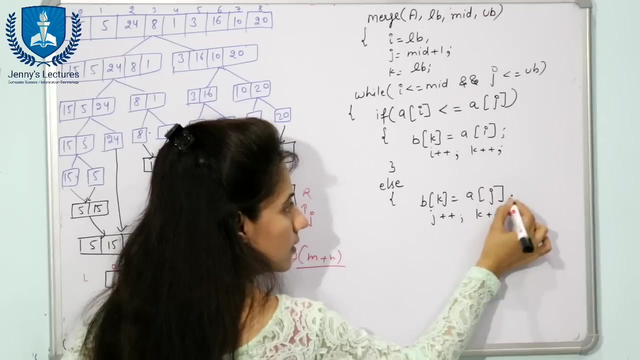 suppose this A of I is not less than A of J, This A of J is less than A of I, Then what you will put, You will put this value into here only So, else what you will do In B of K, you will put A of J, not A of I, And then you will increment J++ and K++. Fine, So. 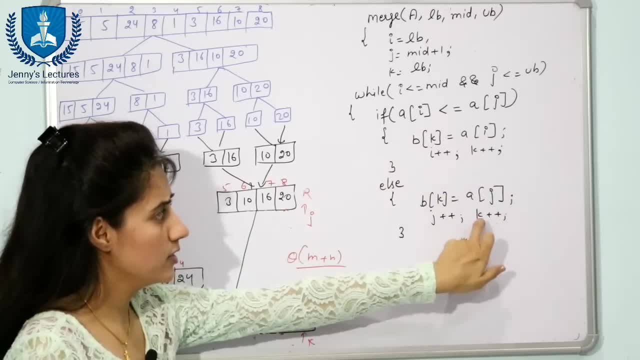 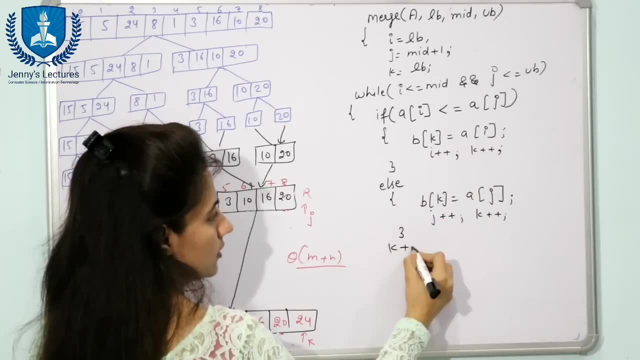 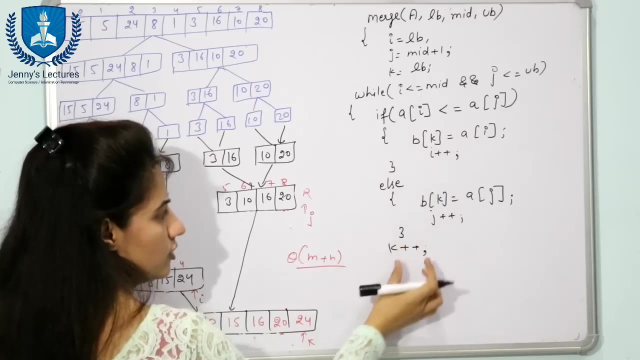 see, in both the cases we have We have done what K++ and K++. So if you will not write here, then you simply write here: K++. You can no need to write here. only You will simply write out of this, if and else. 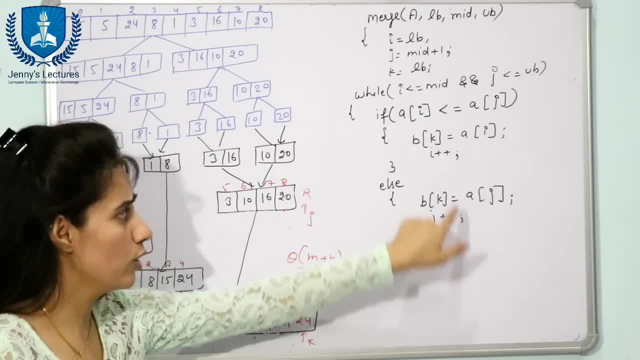 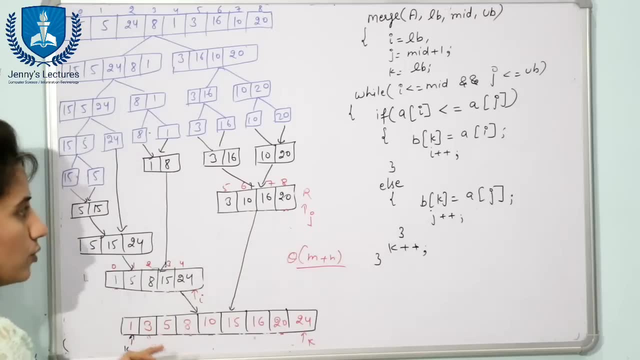 you simply write K++, because in both the conditions you are going to do what K++, K plus one. you can say: Fine, So this is to be this. this procedure is going repeat until we have i less than equal to mid and j less than equal to upper bound. fine, now next. 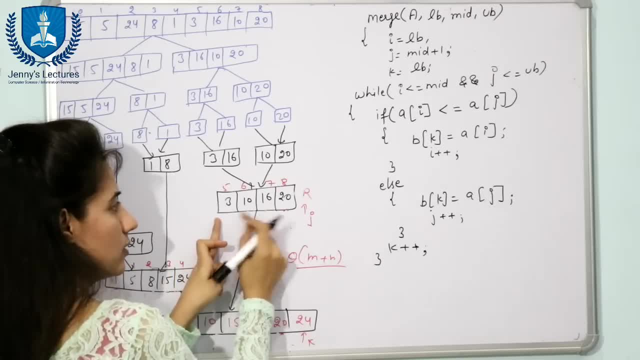 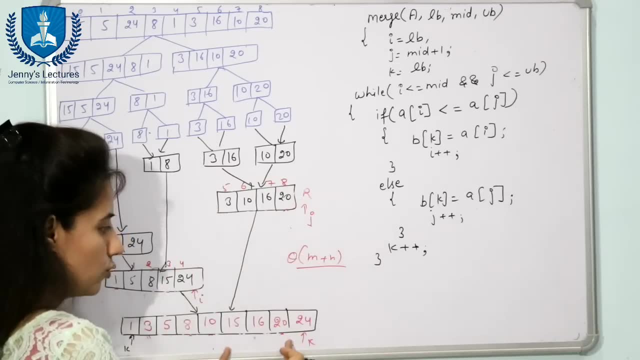 next condition is: what suppose we have reached j is greater than upper bound. now we have already put all the elements of this sub list into this one, but still some elements of this, this sub list, is remaining. then what you will do? you simply put all these elements here, only so you have to check. 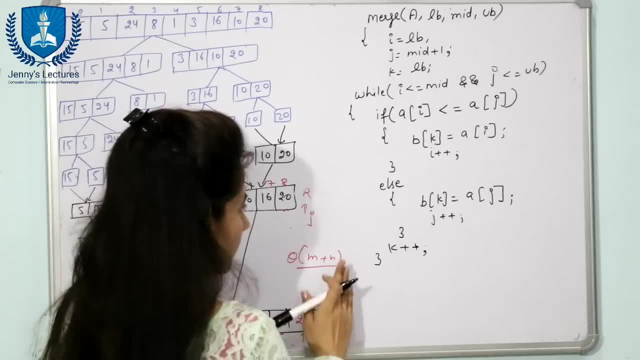 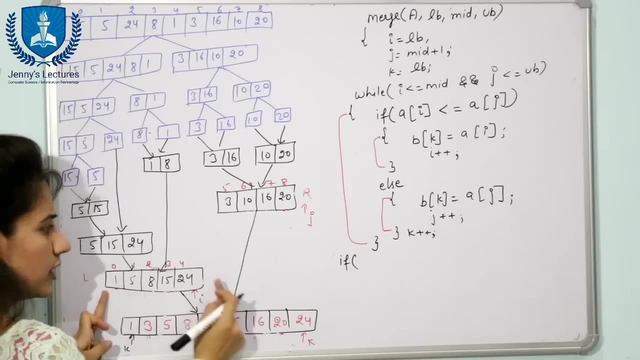 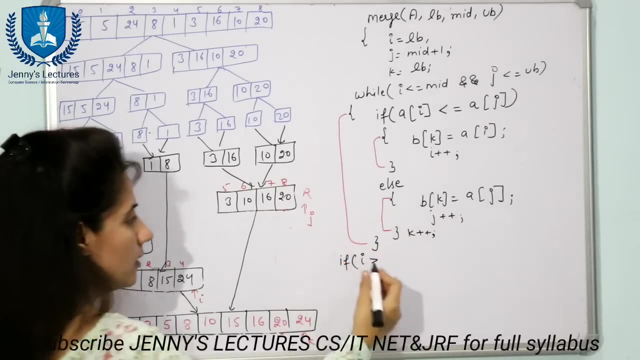 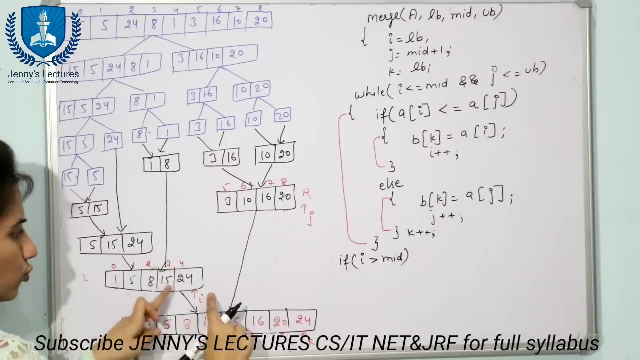 that condition also. fine, now how to check that thing? if now i am going to take, suppose, one condition is i am going to take this, i has been reached to its, beyond, to its limit. so suppose i is greater than mid, because i should be less than equal to mid. now i has been reached to. 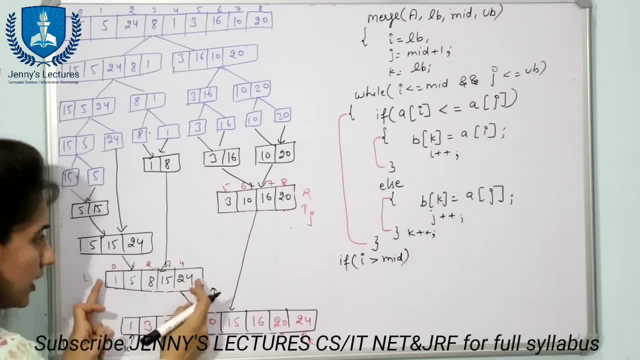 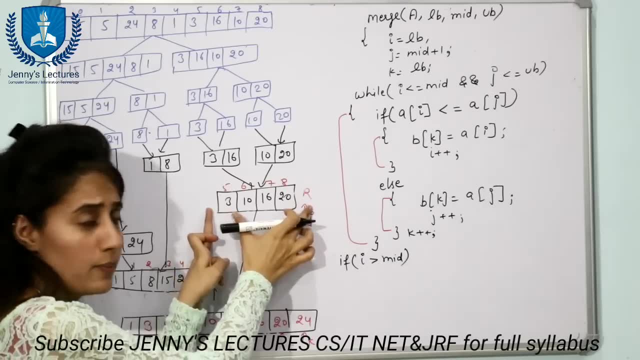 greater than mid means. i has been reached here only. it means all the elements of this sub list has been put here, only now, only some. some elements of this are remaining, may be some elements of this list are remaining fine. so if this condition is there, then then what you will do? you will put now. 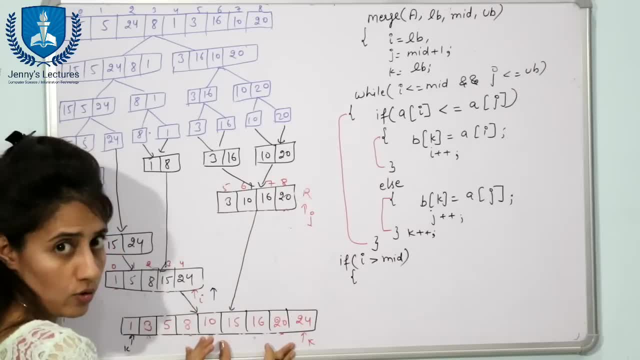 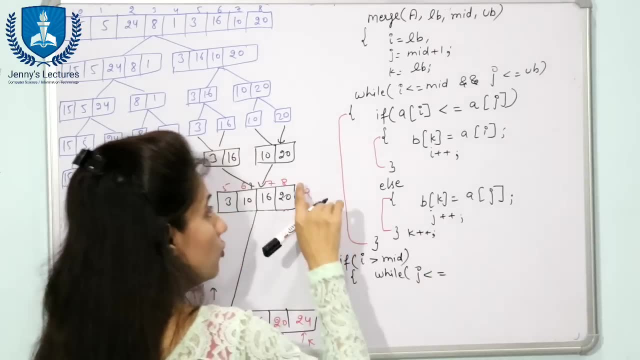 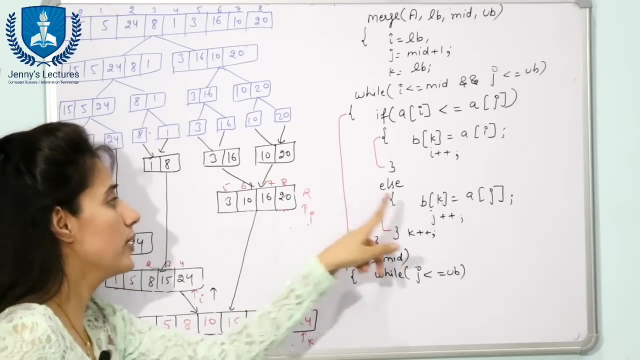 all the remaining leftover elements of this sub list to here only. so now what you will write: while j less than equal to upper bound, while j less than equal to upper bound, only fine, because if j is also greater than upper bound, then no need to. then obviously there is no leftover element. 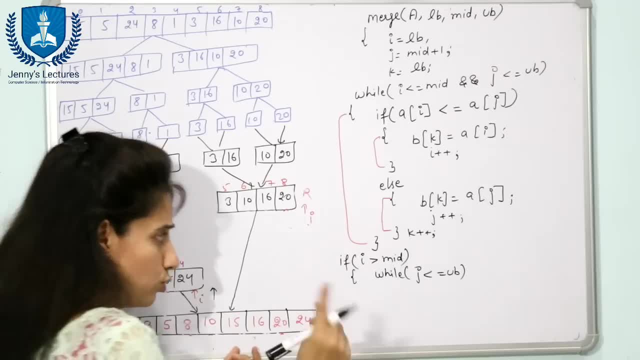 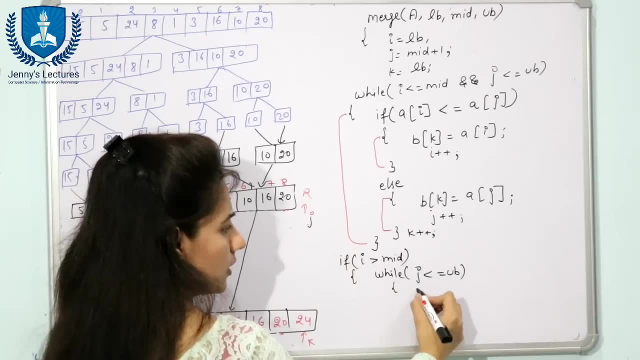 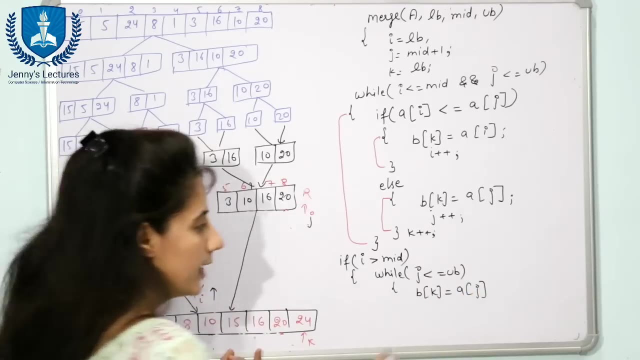 so no need to put these elements here. only. fine, so you will write down that condition also, while j less than equal to upper bound, fine, then only you will put what in b of k, you will put a of j and then you will do what j of j plus plus and k plus plus. 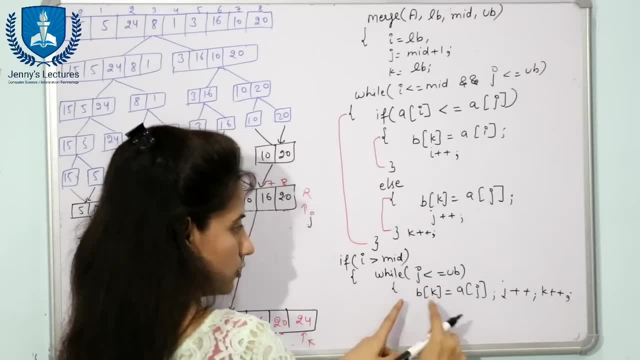 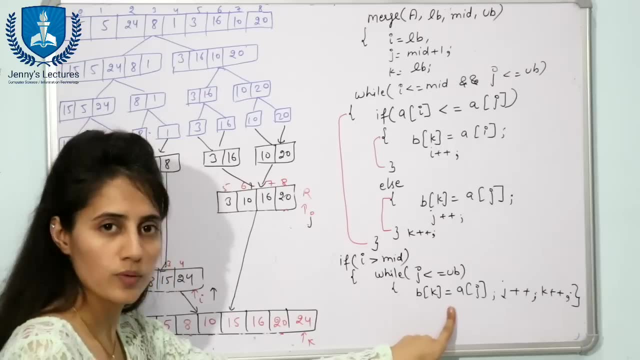 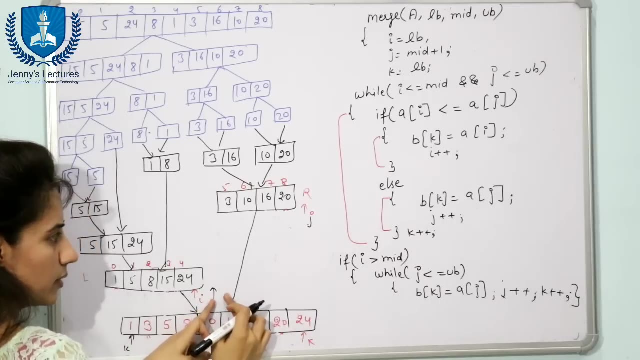 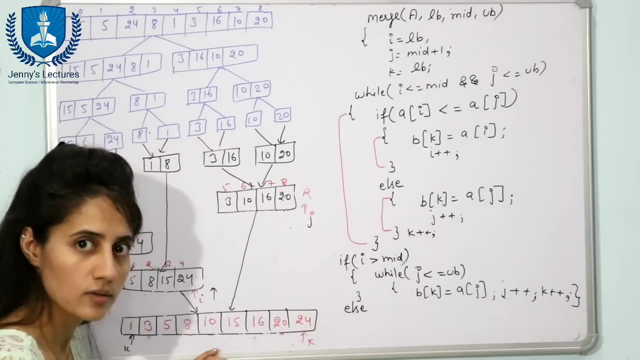 i am short of the space. that is why i am writing multiple statements in one line. fine, and here you will enclose this while loop. okay now second case is there. here i has been reached to greater than this mid. else here, if has been closed, else, if j has, j has reached to its upper bound limit. 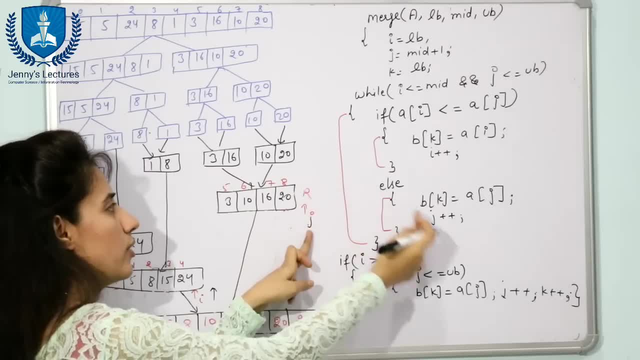 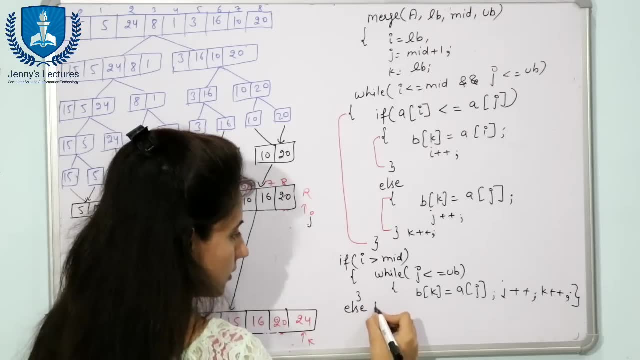 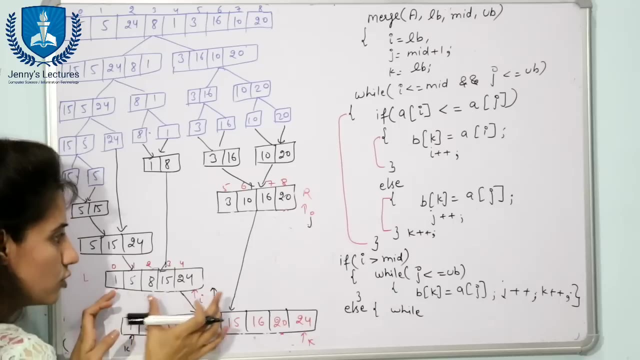 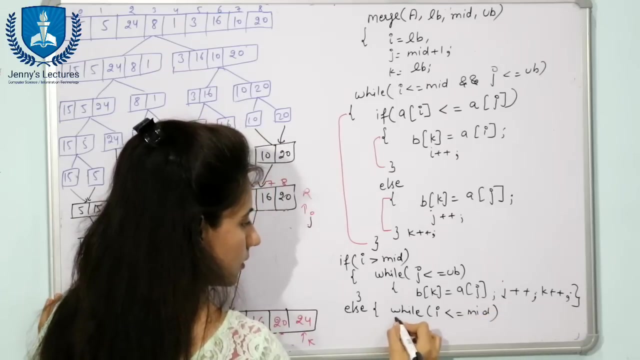 beyond to its upper bound limit, that is, j is supposed now greater than upper bound. so now what you, what you will do. else else you will check. else, maybe some elements, some leftover elements, are there in this sub list, so you will check, while i less than equal to mid, in that case you will. you will do what in b of k you will put. 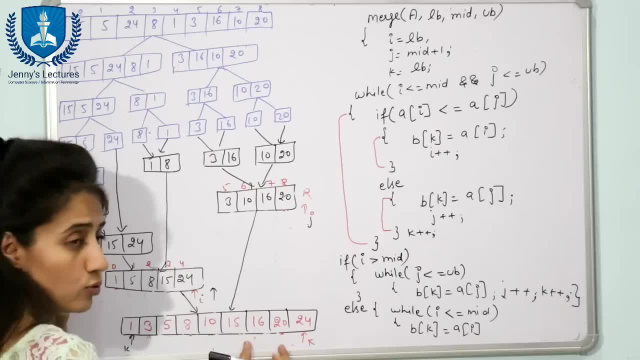 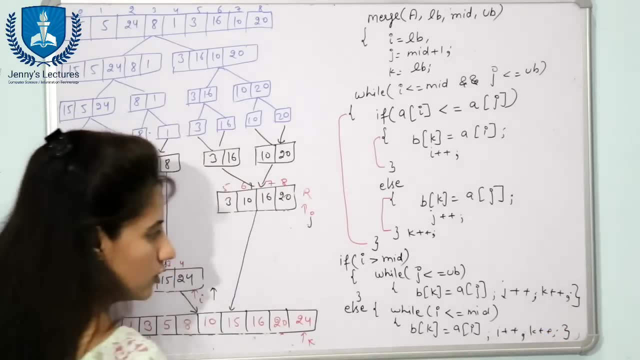 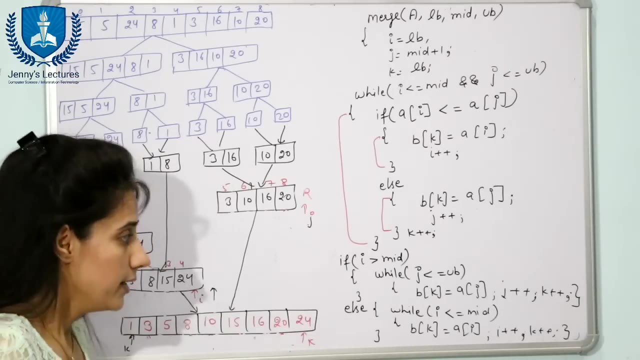 a of that, else you will do what? in b of k you will put a minus theとか i is less than a of i. you will copy all the values here, only now, fine. and you will do i plus plus and k plus plus. this is ending of this while loop and this is ending of this else loop. fine, now see, we have. 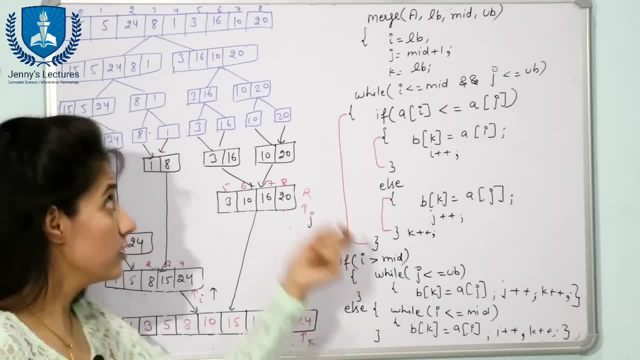 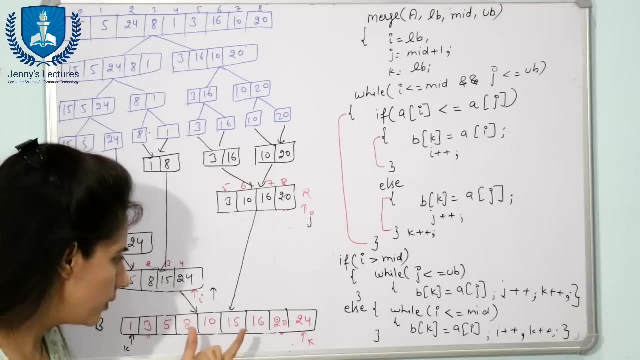 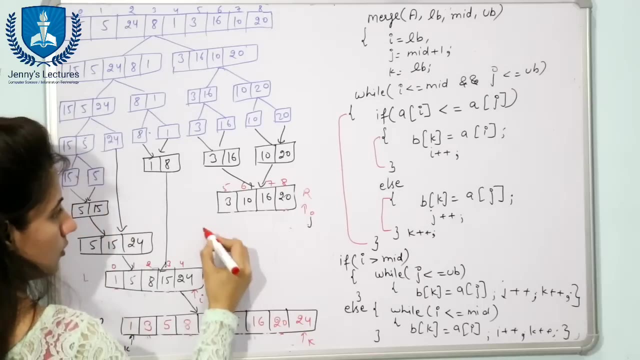 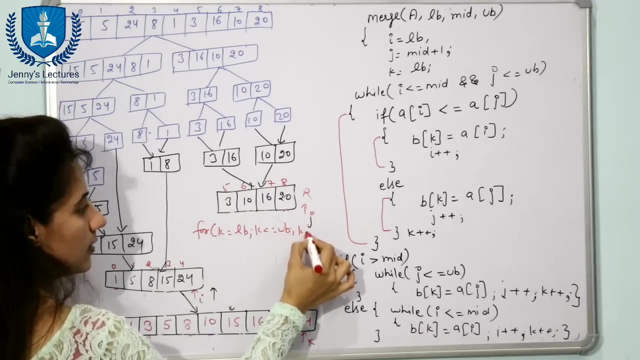 taken another array that is b and the original array is a. so now this b? suppose this is b. so now this is sorted array. you simply copy all these values to this a. simply write down a for loop, for like this: for k is equal to lower bound, k less than equal to upper bound, and k plus plus, and simply copy. 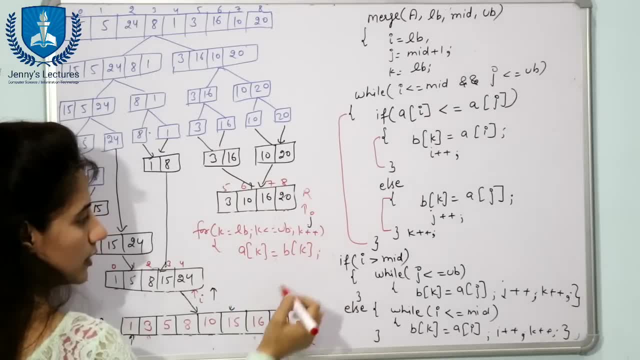 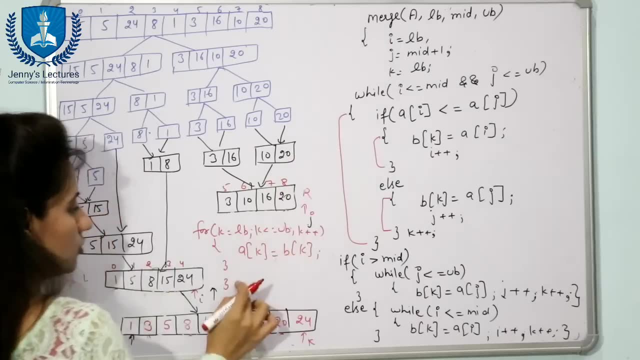 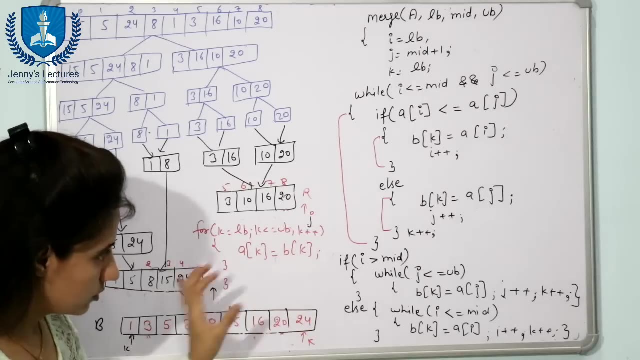 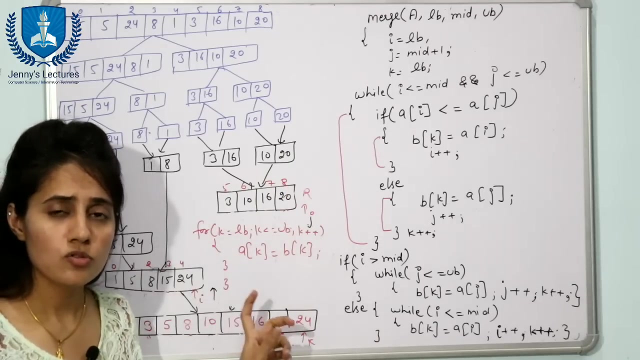 in a of k, you will copy what b of k, all the values from b to a, and this is done now and after that you will close this merge function. ok, i know this is very congested because i have a shortage of the space, but i hope you got the concept of this merge function and the time complexity for this merge. so it is. 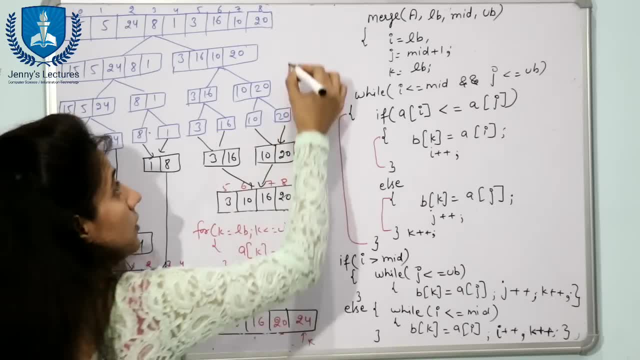 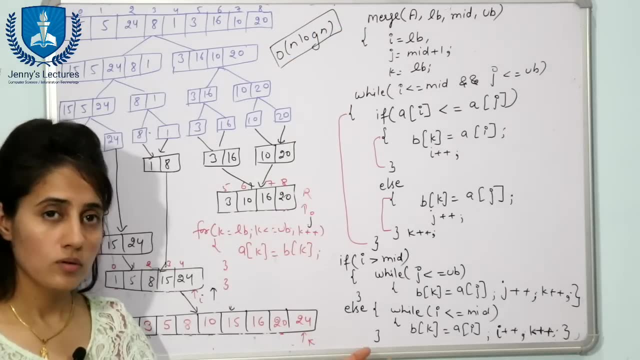 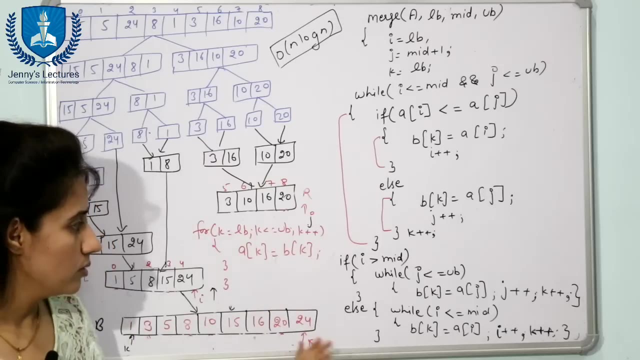 both in worst case and best case it is order of n log n. so i will make another video on this time complexity- how. this time complexity is order of n log n, both in quick sort and merge sort. so this is all about merge sort algorithm. see, if you know the 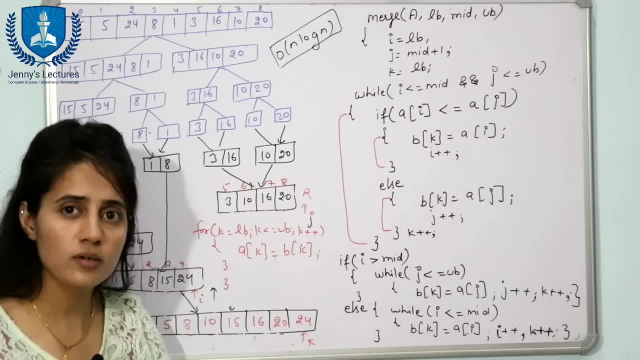 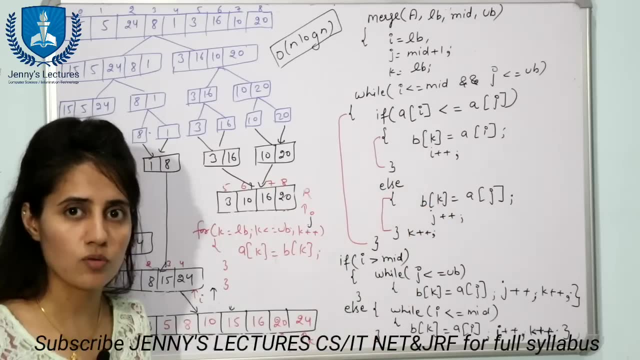 logic of this merge function, then simply, you can easily write down the coding for this merge sort. this is the main funda, this is the main- uh, you can say the backbone of this merge sort algorithm. fine, so this is all about merge sort. in next video i am going to discuss with you.